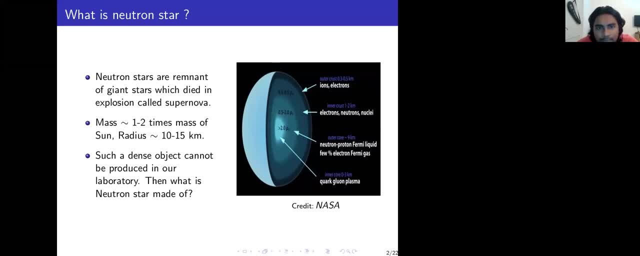 after the collapse they become black hole and starts which are in between 8 to 30 times the mass of the Sun. After the collapse they go through supernova and leave behind a dense material which is known as a neutron star. So the typical mass of the neutron star is: 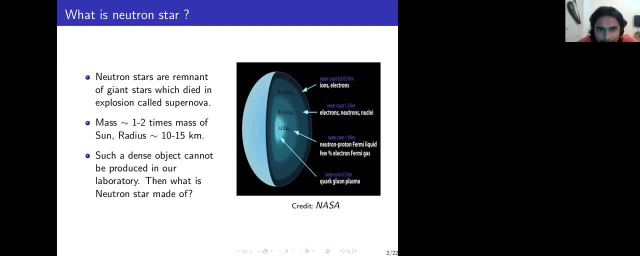 in between one to two solar mass, and it could be more than the two solar mass also. so the exact upper limit of newton star mass is currently not known to us yet, and the radius of a newton star is in in between 10 to 15 kilometers. so if you can imagine that, if you can crush the sun, 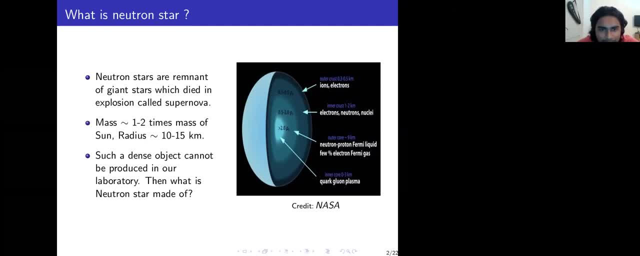 uh, inside a city like kolkata. so this will be our neutron star. so uh that, and so you can. so you are currently understanding that the new cluster would be very dense object. so if we take, for example, if you take, one spoon of material from neutron star, it would weight the same as 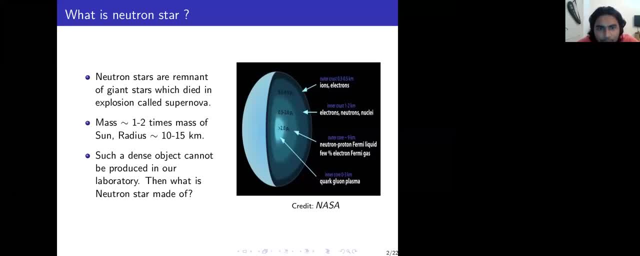 mount everest. so therefore, the fundamental question is: what is new cluster made of? so here in the right, i have shown you a schematic diagram of newton star. so the current understanding is that newton star possess a crust which is of the order of one to two kilometer. 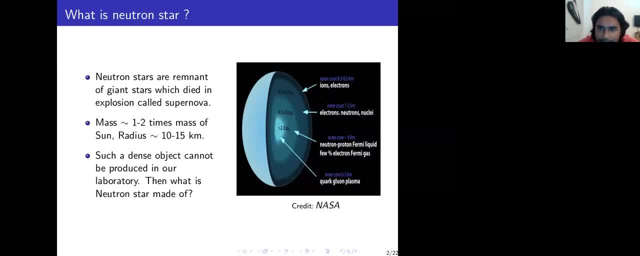 and inside the crust nuclei are arranged in a lattice form, and as we go from surface to center of the neutron star, the density increases rapidly. so, for example, at the surface of the neutron star uh the density is of the order of 10 to the 6 gram per centimeter, and at the center of 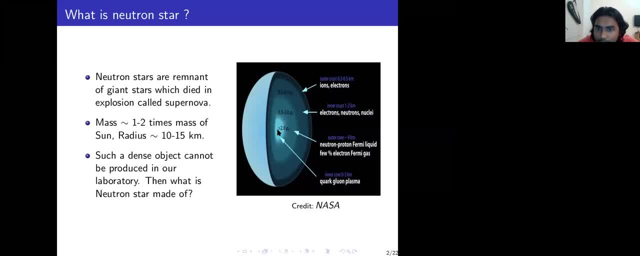 the neutron star density could increase up to 10 to the 16 gram per centimeter and as we go from surface to the center, the neutron uh, the density of the nuclear matter increases and in the inner outer color core of the neutron star there will be homogeneous nuclear matter and the inner core of the neutron star some exotic. 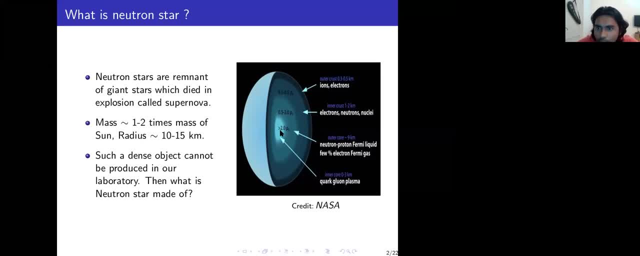 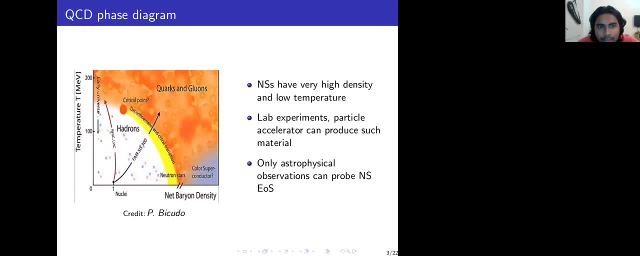 material could appear like uh quark, uh hyperones. those may appear now the. the question is: can we make uh a new cluster type of material in our lab? so to understand this, let's see this diagram which is between: between uh temperature versus the net variant density. so the normal material which we observe in our 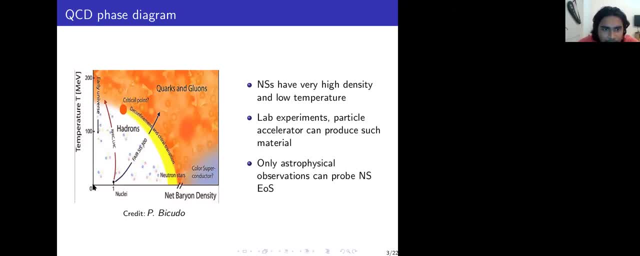 earth or which we deal with in our lab experiment. those lies in this region where the temperature is low. as well as the number, density is also low, and this is the normal nuclear density, which is also known as the nuclear saturation density. also now, in order to go to the high density, 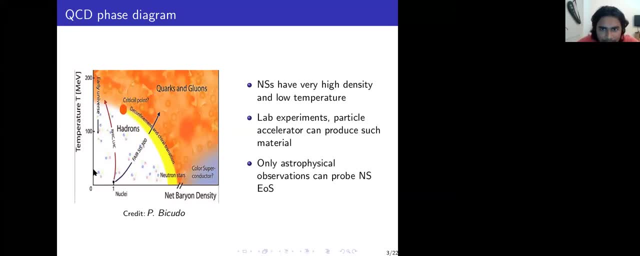 we have built particle accelerator. so in particle accelerator we can raise the temperature of the atom verticalід brunch gradient to the components, to u library. we have some different capable to achieve that, in which we see in normall ways, you see the temperature and go to the high density also. So here for example, particle accelerator. 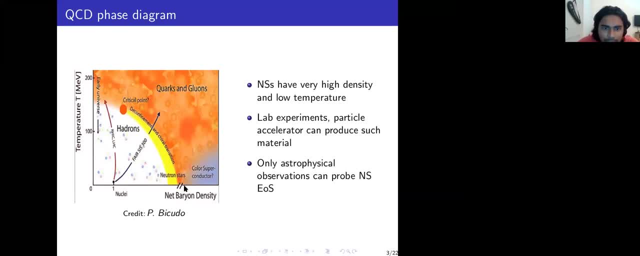 they do operate in this region, But Newton star. they lie in this region where the density of the Newton star actually five to six or could be up to 10 times higher than the normal nuclei, But they also have very low temperature. So low temperature means their temperature. 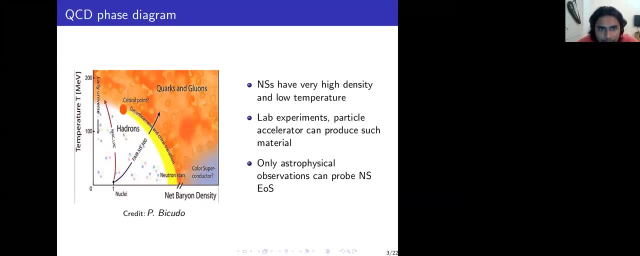 is much more lower than the Fermi energy level. So from this diagram it is clear that we cannot make new construct type material in our lab and as well as also with the particle accelerator. Therefore, the only way we can probe Newton star using the astrophysical observations. 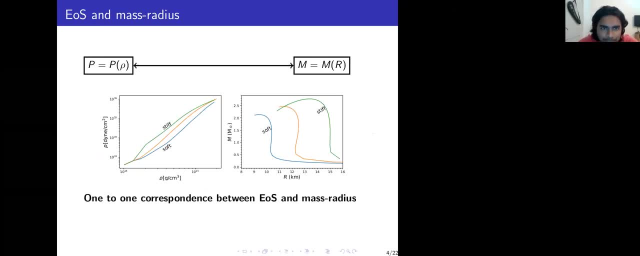 Now let's talk about the Newton star equation of state and the mass ideas. So Newton's equation of state is the relationship between the pressure and the energy density inside the Newton star. So this is the equation, the expression of the equation of state. Now 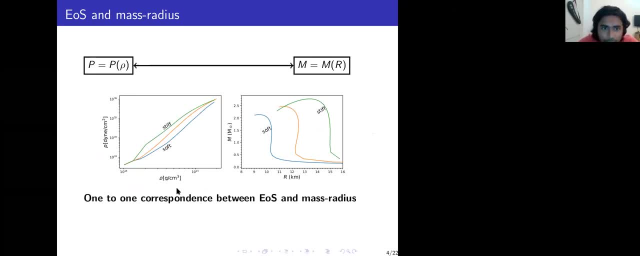 here diagram. I have shown you three different type of equation of state. The bottom one is the soft equation of state, and for the soft equation of state we see that the energy density, the pressure, increases less rapidly with the energy density. and the upper one is the steep equation of state. 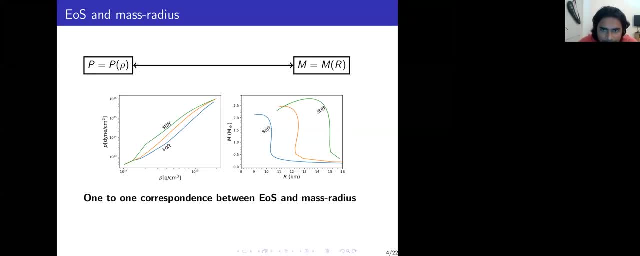 for which pressure increases more rapidly with the energy density. Now, given these three equations of state, one can ask: if these are the true equation of state of neutron star, then what would be the macroscopic properties of the neutron star, such as what would be the mass? 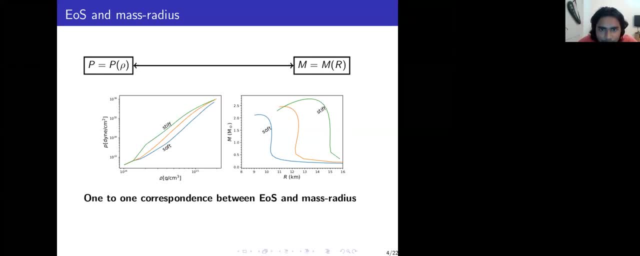 and radius of a neutron star. So to find out that cosine one need to solve the hydrostatic equilibrium equation of for neutron star. So in hydrostatic equilibrium the neutron degenerative pressure will be balanced by the gravity. and if one solve that hydrostatic equilibrium equation, 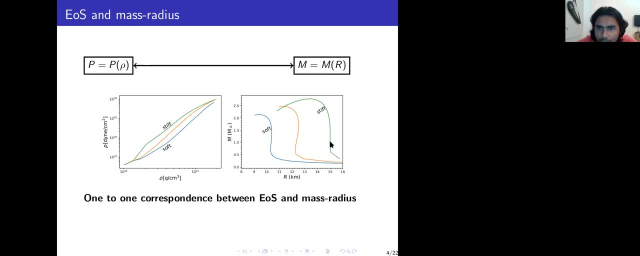 given this equation of state, then we arrive to this diagram, which is the mass radius diagram. So here I would like to point out that this is not a profile, this is a sequence. that what does it mean by that? that means here, each point in this line is a neutron star. Suppose, if we take 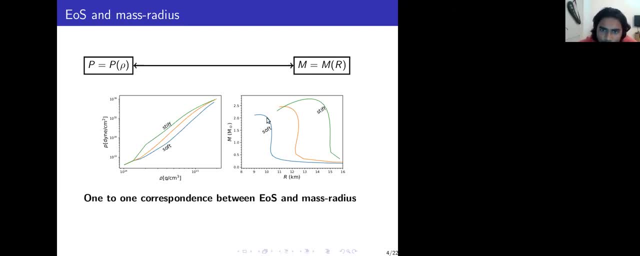 this point here. this is a neutron star which has a mass around two solar mass and the radius around radius around 10 kilometers. Okay, so now for each equation of state. here one thing is noticeable: that for each equation of state there is a maximum mass. So for this equation of the maximum mass lies, 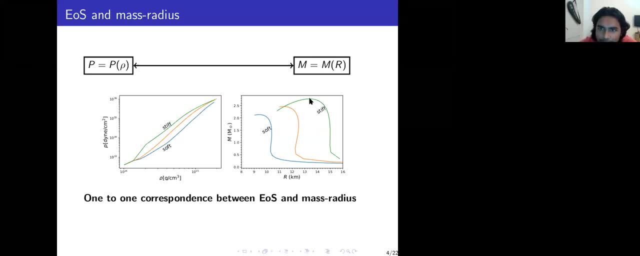 around here, or this equation of state maximum mass is around here and as we go from the soft to steep equation of state, the maximum mass actually increases. and the other thing is noticeable that the for the steep equation of state radius is also higher compared to the soft one. 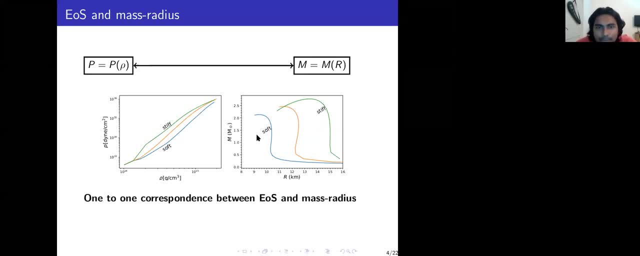 Now the question is: which one is the correct equation of state? so that answer is: we do not know, because we do not know what is the correct constitutive state of Newton star. And even if we guess the materials inside a Newton star, we do not know. how do. 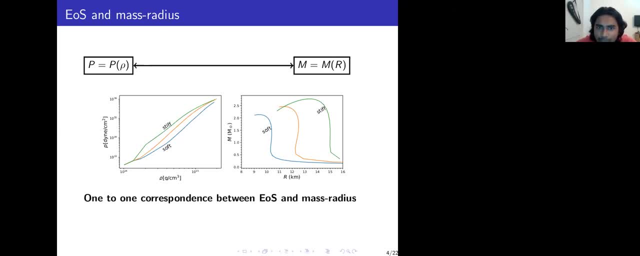 they interact in that high density. Therefore, we come up with some models and those different models leads to different equation of sets. So, for example, you are seeing three different kind of equation of set And for those equation of three different equation of set, the mass. 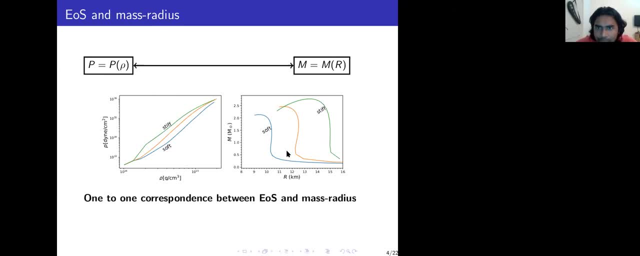 radius relation are also different. So the idea is, from the astrophysical observation we will be observing many, many Newton star. So one Newton star, let us say, will be here, then another Newton star will be here, then here and so on. So when we will have many, many 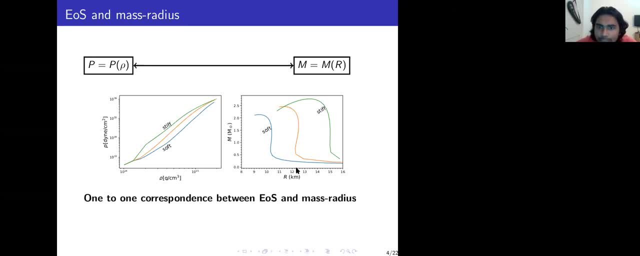 Newton star observation, we will connect those dots and we will get this mass radius curve here. And since this mass radius and the pressure density has one to one corresponding with each other, so from this curve we can go back to this curve and we can know the what is the correct. 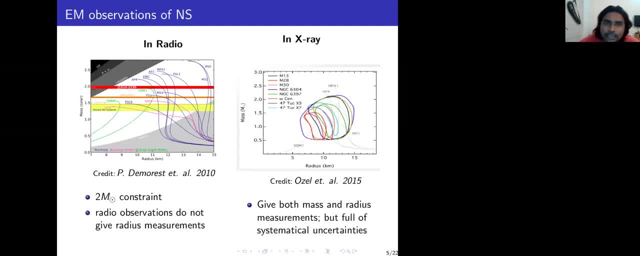 equation of set of Newton star. Now let us talk about the observations. So Newton star are observed in different different electromagnetic bands. So it was first observed in radio. So it was a lady, her name is Jocelyn Indale. Actually, she observed the radio pulsar for the first time when she was a grad student at 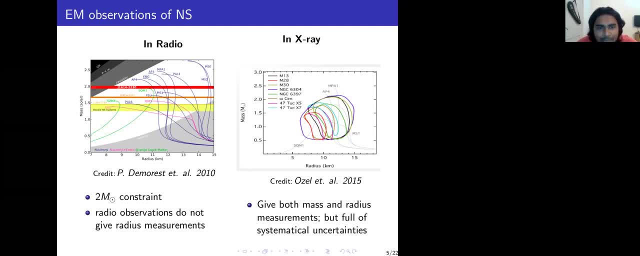 Oxford, But unfortunately her supervisor took all the credit for discovery and he got awarded the Nobel Prize. But later we came to know that in 2018, later we came to know that actually she is the one who found, who discovered, Newton star, and in 2018 she has been awarded the breakthrough prize. 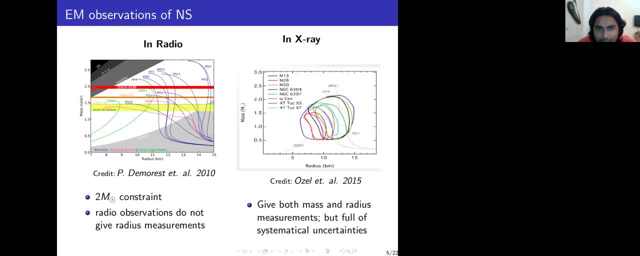 But she donated all her money which she got from the breakthrough prize for the women's science. So this is a bit sad story, but a motivating one also. Now from the radio observation we find the mass of the Newton star very accurately and we have observed few massive Newton star. So here 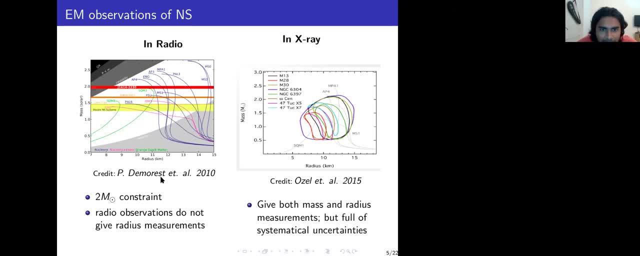 I would like to point out one particular observation: that that has been done in 2010 and we have observed a Newton star which has marched around 1.97 plus, with a lower part of plus minus 0.04.. So that is shown here by this red band. Now this observation actually helps. 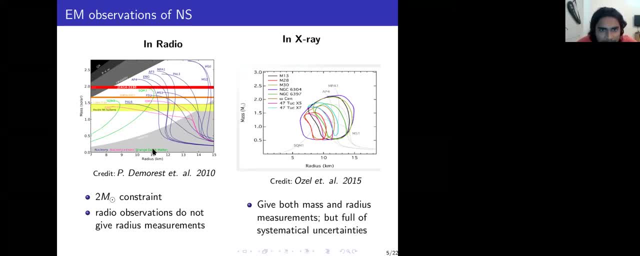 us to rule out many equations of state. So you can see there are many equations of state which cannot reproduce that two solar mass neutron stat, For example here: MSO1, FS2, GM3, TAL6, GS1,. 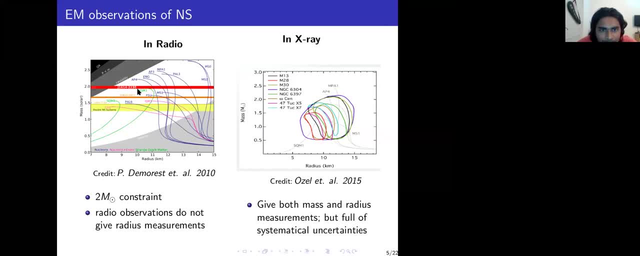 those equations of state. they are unable to reproduce that kind of maximum mass of a neutron stat, So they are automatically ruled out now by this observation. But still we are left with many equations of state which are shown here. Now how to discriminate between those equations of state? 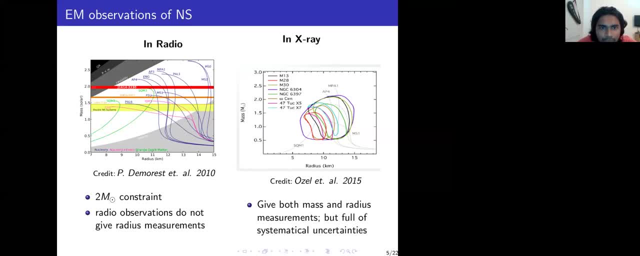 To discriminate between those equations of state. we need also radius observation. But unfortunately radius observation do not give us radius measurement, but X-ray does. Now in X-ray we observe neutron star in a binary neutron star system. Those are called low-mass X-ray, binary neutron star system. 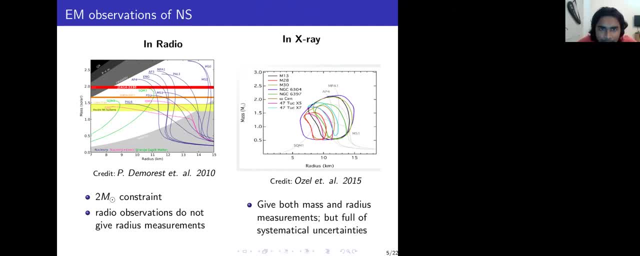 And in a low-mass. in that type of system, actually neutron star accretes matter from the low-mass star and because of the accretion an accretion disk is formed around the neutron star. And when the accretion disk gets luminous, 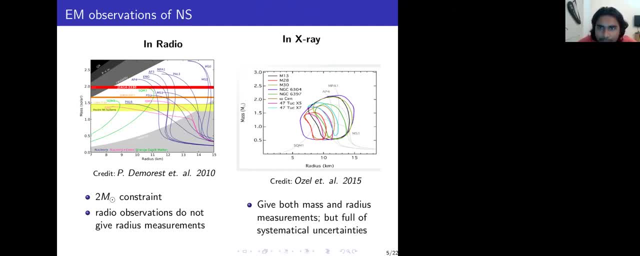 we can actually observe through our X-ray telescope, And from the luminosity of that X-ray we can determine the mass of the neutron star And also from the spectra we can determine the radius of it. So here I have shown you some X-ray measurement here. 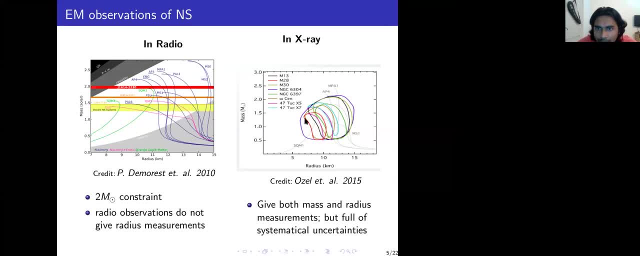 So here each contour actually signifies one neutron star observation. So earlier I talked about that. from the astrophysics we will be observing many, many neutron star and that will be a dot in the mass of the neutron star Instead of a dot. you can see that we are getting a contour here. 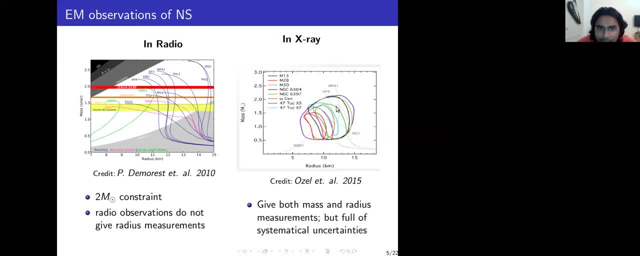 because astrophysical observation do have some lower bar. So instead of getting a line in the mass of the neutron star, we'll be getting a band in the mass of the neutron star and also as well as in the pressure density plane. Now X-ray observation have some systematic uncertainties. 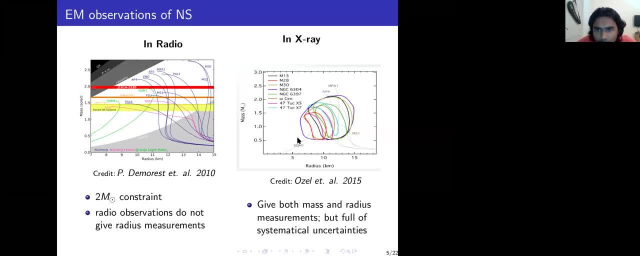 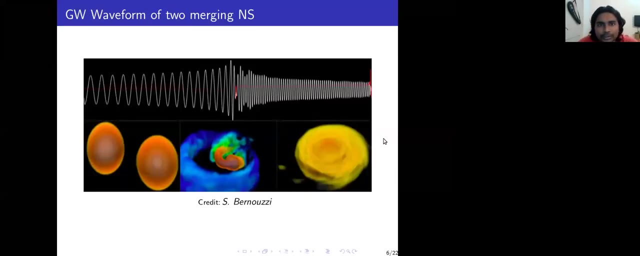 because in order to determine the radius, we need to model the atmosphere of the neutron star accurately. but that is also model dependent, So that model dependency actually increases some systematic uncertainties. Now let's talk about GW observations. So, as you know that in 2017, 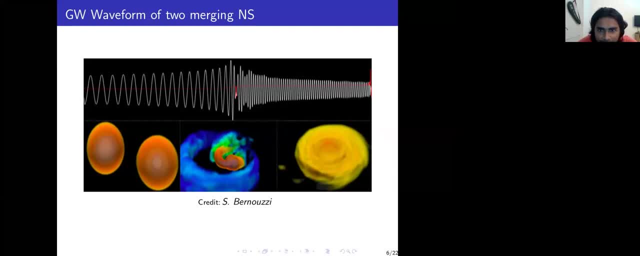 LIGO-Vargo collaboration. for the first time they discovered gravitational wave merger from a binary neutron star system. So here in this schematic diagram I show you different phases of binary neutron star. So here in this schematic diagram I show you different phases of binary neutron star. 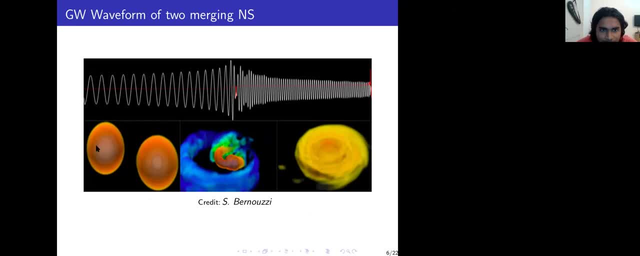 So here in this schematic diagram, I show you different phases of binary neutron star. So this one is called the inspired phase. So inspired phase when two neutron stars, they are rotating around each other and as they are rotating around each other they emit gravitational wave. 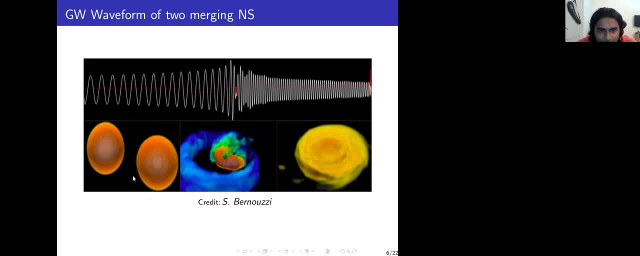 Since they are emit gravitational waves, the system is loosing energy and the whole bit trends. Since they are emitting gravitational waves, the system is loosing energy and the whole bit trends. At some point they merge with each other. So here the merger scenario you'll find: 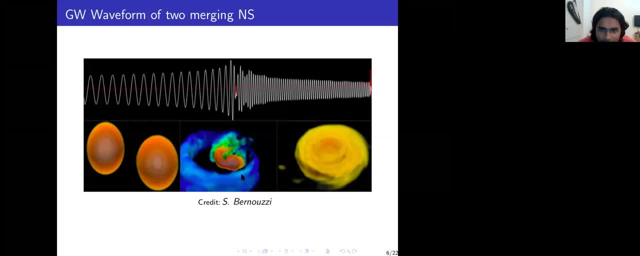 and this merger scenario is a bit complicated, because the sacrificial themselves called the harmed energy: weil wir machen das alle einen enrichen den bekommen. During the merger a lot of materials will be ejected, those are shown here by this color, And after the merger actually a single body is formed and that body will be highly rotating. 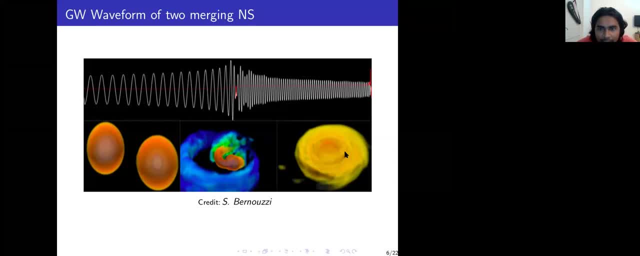 object and as well as also oscillating object, And during this whole phase actually the gravitational wave is emitted. So here the gravitational wave form is shown as a function of time. So as we approaching from the inspiral to the merger, you can see the frequency actually. 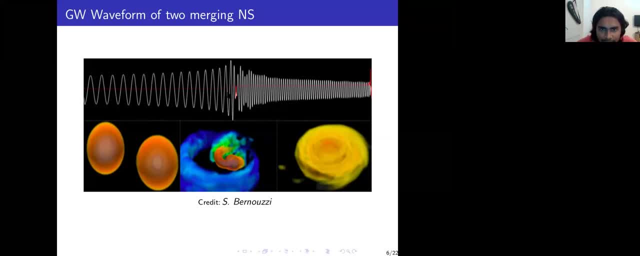 increasing and as well as the amplitude also increases, And at the time of merger actually the amplitude is maximum. And after the merger- this is called the post-merger phase- still we see gravitational wave emission. as long as this body rotates, and as it stops rotating, this emission will be stopped. 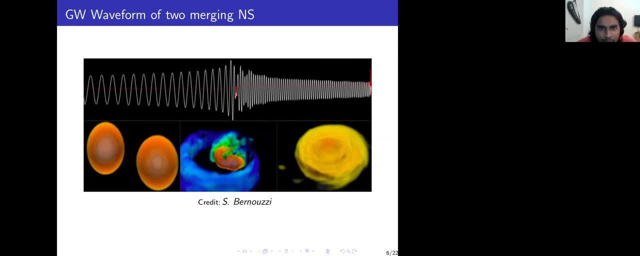 Now, LIGO-FALCO instrument is actually sensitive to the frequency And it observes a particular frequency. It observes a particular part of this waveform. So LIGO-FALCO instrument is actually sensitive within the frequency range of 20 Hz to 1 kHz. 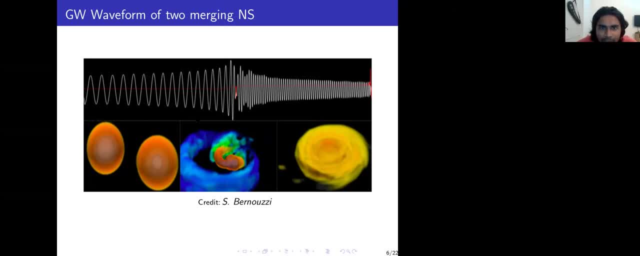 And that frequency range actually covers this inspiral part only. So with LIGO-FALCO we cannot observe the merger phase and as well as the post-merger phase, because the frequency is higher in those phase. So now we have to do fundamental analysis. 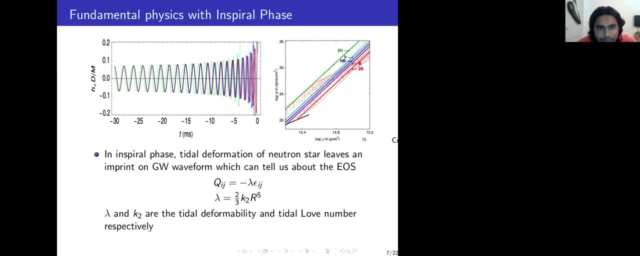 Okay, So we have to do fundamental physics with the inspiral phase. So the question is what type of fundamental physics we can do with it. Now, when two lintels stir, they rotate around each other. in an inspiral phase, they get tidally deformed because of the expansion. 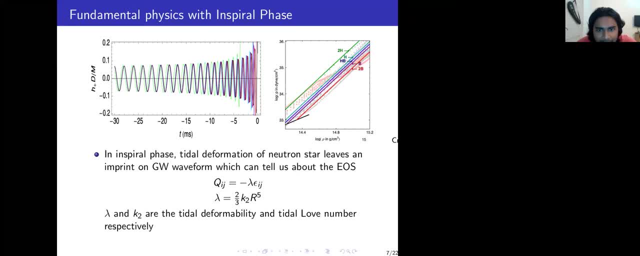 Now, if we are looking at a spiral, we have to do an unbalanced regression. So this is the unbalanced regression. So basically, this is a hook slow type regression, So the stress is proportional to strain The single thing. you can find the analogy from here. 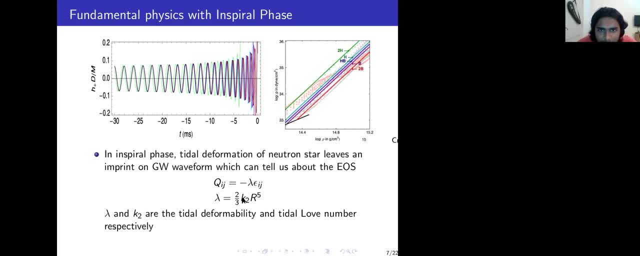 because this enters in the phase of the gravitational wave. Therefore it can modify the gravitational wave signal. So here in this left plot you can see the magenta color is plotted here without the tidal deformation And the green one is plotted with the tidal deformation. 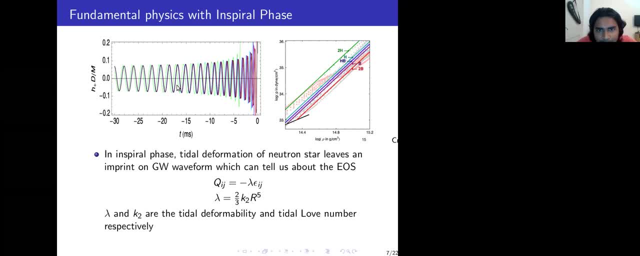 So you can see there is a mismatch in phase And from the observation actually, we can find out the mismatch in the phase and we can calculate what is the value of the lambda. And this lambda depends on the equation of state of the neutron star. 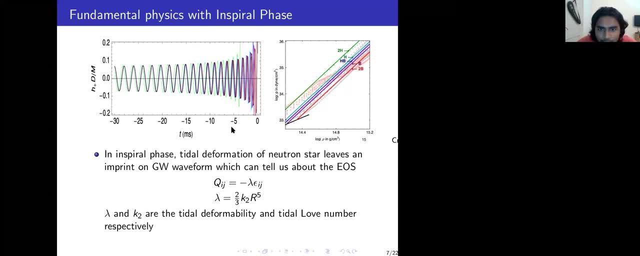 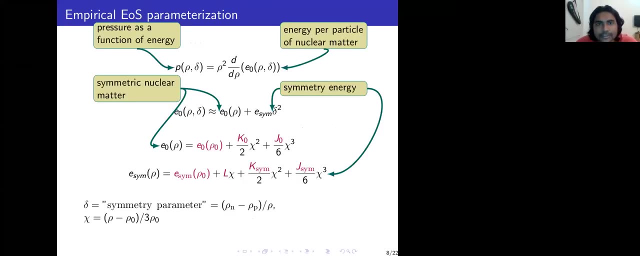 It depends on the mass and radius of the neutron star. Therefore, through the measurement of lambda, we can constrain the equation of certain neutron star. So we can go from this plot to this plot. Now, since we're interested in constrain the equation of state of neutron star, 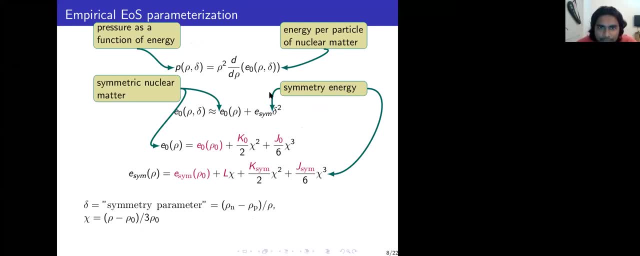 let's talk about how to parameterize the equation of state of neutron star. So here the top equation is the expression for the equation of state, which is a relation between the pressure inside a neutron star And E naught is the energy per particle of a nuclear matter. 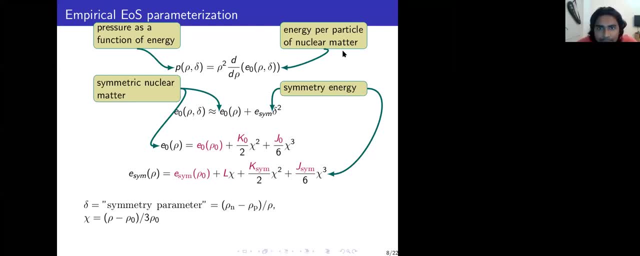 Now, inside a neutron star, matter is asymmetric in neutron to proton ratio. So therefore one can split this term E naught in two terms: one for the symmetric neutron matter, which is this E naught rho, And another for the asymmetric neutron matter. 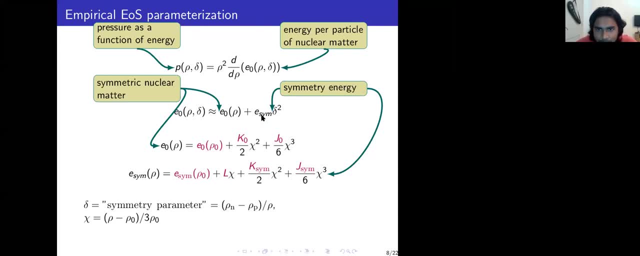 which is this term. So this term is known as E naught, denoted as eSIM here, and this is also called the symmetry energy. So that signifies how symmetric or asymmetric the neutron matter is. And delta is our symmetry parameter, which is defined at the bottom of this slide, So which is equal to rho n minus rho p by rho. 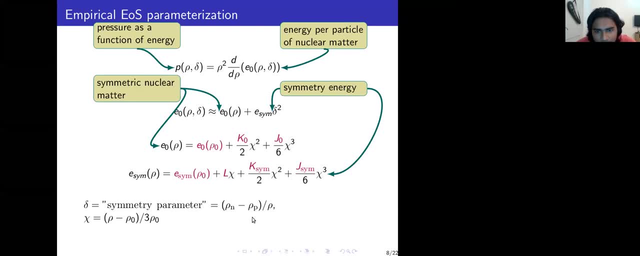 where rho n is the number density of the neutron and rho p is the number density of proton and rho is the total number density, that is, rho n plus rho p. Now we go a little bit further from this expression and we expand these two terms in a Taylor. 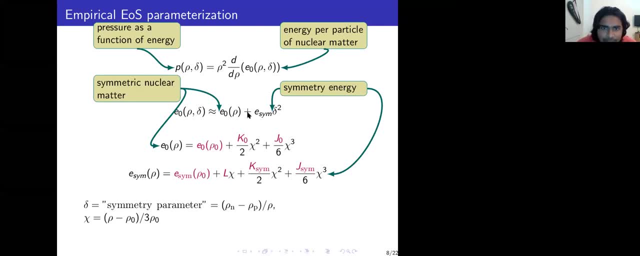 series about the nucleus saturation density, because about the nucleus saturation density these two terms have a minimum and we keep up to the quadratic term here and while expanding in a Taylor series we get few coefficients. So those coefficients are shown here in magnetic color, so that E0, K0, J0, eSIM, L, kSIM and jSIM. Now these are the parameters of our 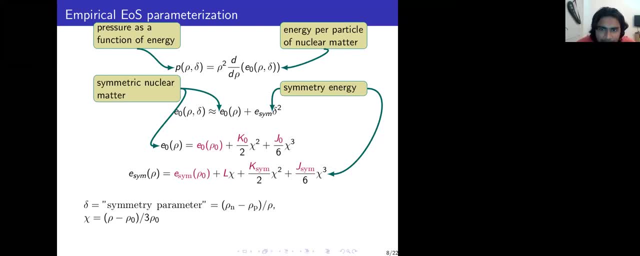 model. These are the parameters of our model Now. these are the parameters of our model. So these are the parameters of our model. So these are the parameters of our model model now, and this constitutes the parameterization. So our target is to constrain these parameters. 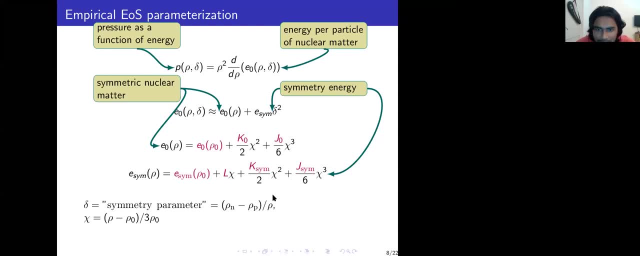 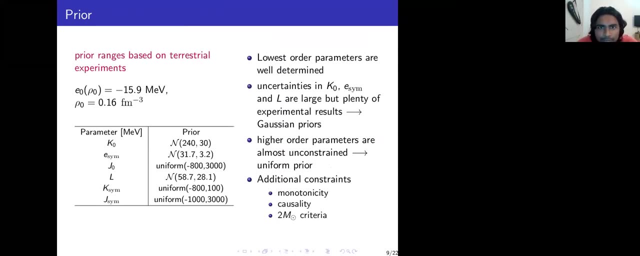 from astrophysical observation, And when we get those parameters from the observation we can put constraint on the equation of state of infrastructure. Let's talk about the priors. So here priors means whatever the prior knowledge is we have about the nuclear parameters. 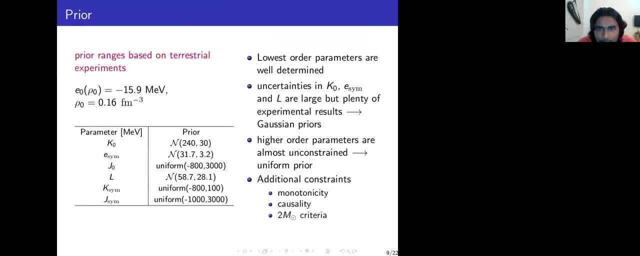 So for that we divide our nuclear parameters in three class. In one class there is the lowest order parameters, which are E naught and rho naught. So these are the two parameters. So E naught is the binding energy of a nuclear 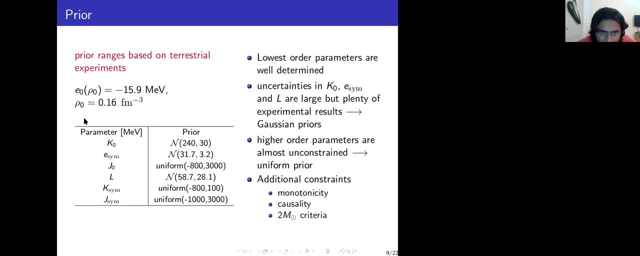 and rho naught is the nucleus saturation density, And from the nuclear physics experiment we actually know the value of this quantity very well. So that's why we fixed them in our study. And the second or next order parameters are K, naught, E, sim and L. 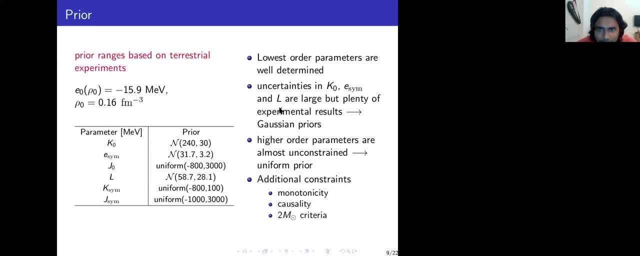 So these parameters are not very well constrained from the nuclear physics experiment. but we have a lot of experimental results and as well as theoretical ab initio calculations. So that's why for those parameter we choose a Gaussian priors, So the value of the median and sigma 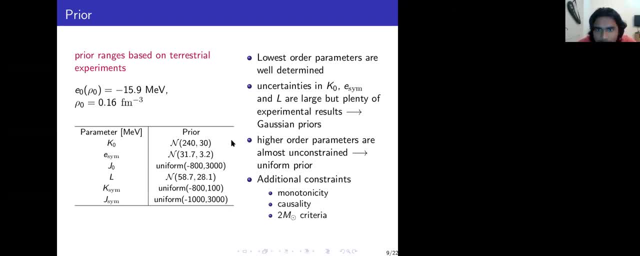 for those Gaussian priors are given here in this table And the higher density parameters are J naught, K sim and J sim, And this prior parameters are given here in this table. So these parameters are not at all constrained by the nuclear physics experiment. 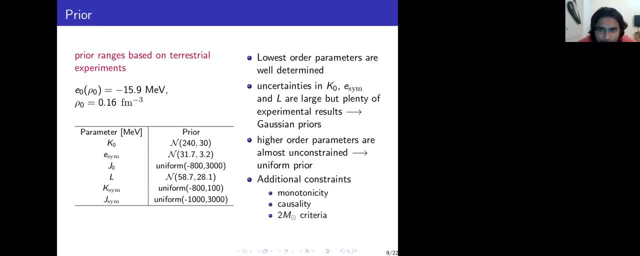 because we cannot reach to that higher density. So those parameters can only be constrained using astrophysical observations only. So that's why we chose a broad, uniform prior for those parameters. Now, additionally, we put three other constant constraints on the Newton's equation of state. 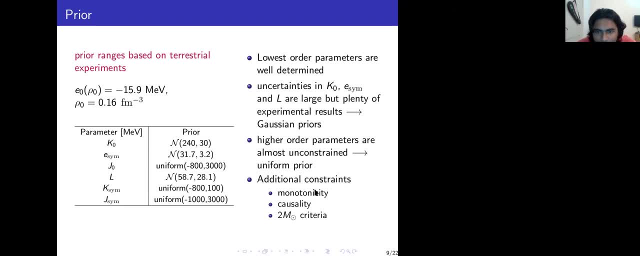 The first one is the monotonicity. That means pressure should always increase as a function of energy density, Otherwise mechanical stability inside an infrastructure will be violated. Secondly one is the causality, So that means the pressure, the speed of sound. 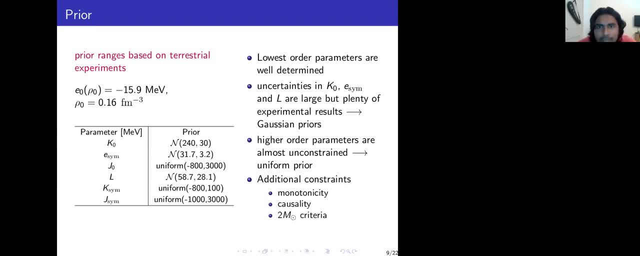 should be much, should be less than the speed of light. So speed of sound is defined as the dp zero, And actually this is the square of the speed of sound, So it can be obtained from the slope of the equation of state. 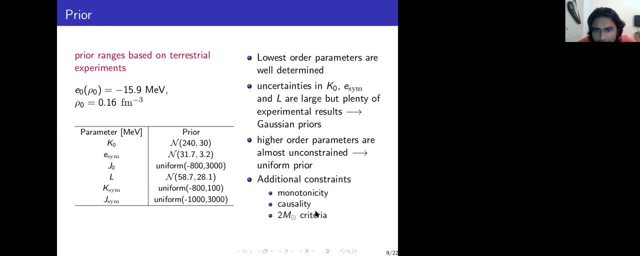 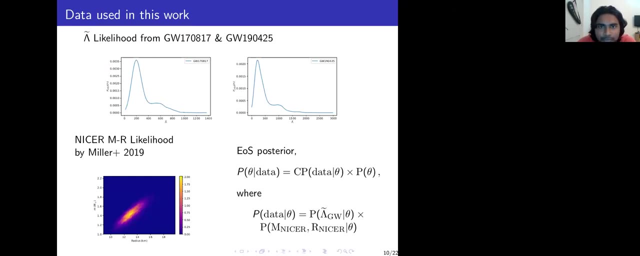 And the two synonymous criteria which you have obtained from the radio observations. So those equations of state which cannot reproduce these two Newton's stat, they will be discarded. Now let's talk about the data here and which we will be using in our paper. 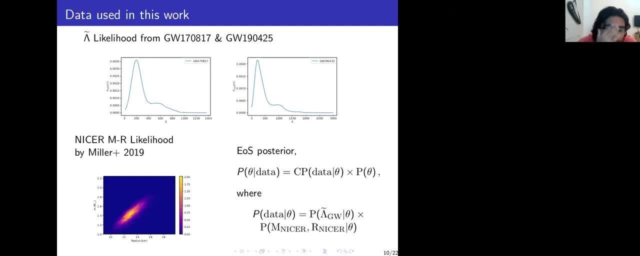 which we have used in our paper. So in our paper we use two GW detection. So first one is the GW17017, and the second one is GW190425.. So let's talk about the nomenclature first. So the first 17 starts for the year. 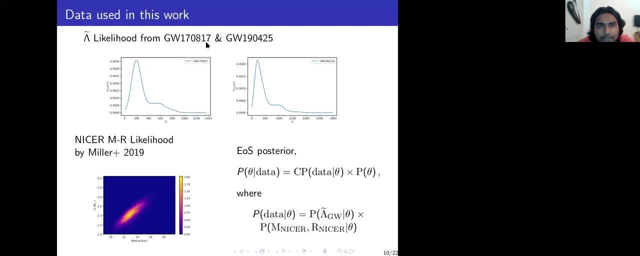 and the second two stands for the month and third, two stands for the date. So this event was observed in 17th of August 2017.. This was observed in 25th April 2019.. So, from the GW observation, 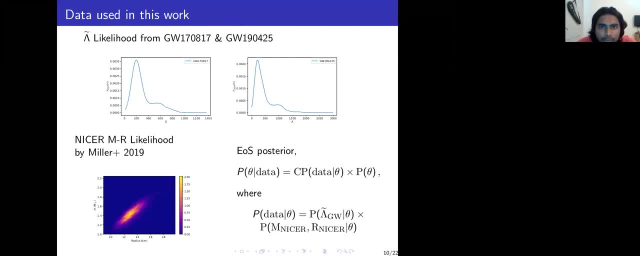 actually the information of equation of state comes through a quantity called lambda tilde. So this lambda tilde is function of mass one mass two. lambda one, lambda two. So mass one, mass two. lambda one, lambda two. So mass one, mass two. lambda one, lambda two. 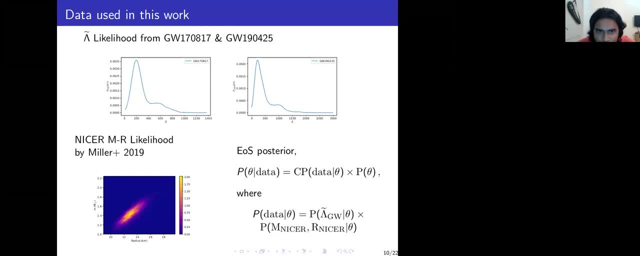 So mass one, mass two are the masses of the two Newton star in a binary system and lambda one, lambda two are the corresponding tidal deformities And these are the distribution of lambda tilde we are getting from the GW observation. So this one is for the first observation, GW17017,. 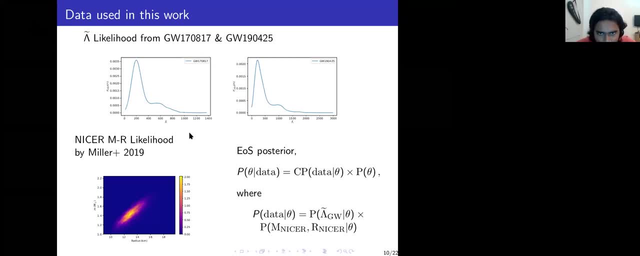 and this one is for the GW190425.. Now, one interesting feature is that this lambda tilde distribution has bimodulating in it. Now, one interesting feature is that this lambda tilde distribution has bimodulating in it, though. so one peak is for 70 to 70, there is one peak around 200 and another peak is around 600.. 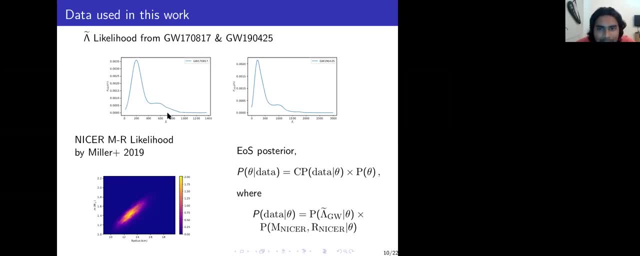 So I'll request you to remember this feature of lambda tilde, because that is going to be important in NASA And recently the NICER mission, which is led by NASA. they have also provided and a very accurate information about the mass radius measurement of a particular 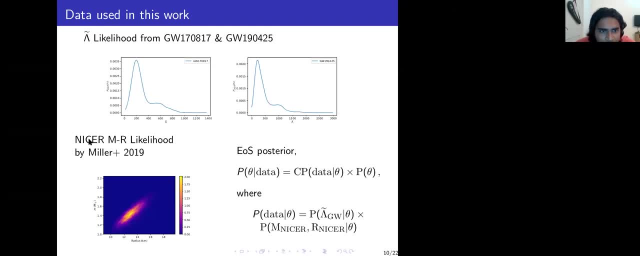 event. So this NICER, the full form of NICER, is Newton star interior composition explorer. So this is led by NASA. So they observe Newton star in x-ray and this is the first time actually they have overcome the systematic uncertainty in their analysis and the 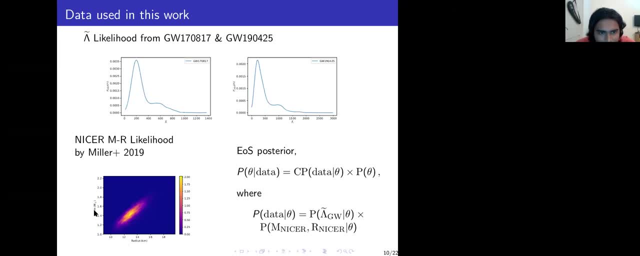 measurement we are getting here is very accurate. So the mass radius distribution for this particular event is shown here in this plot. So the most likely value: you can see from this plot that the radius is around 13 kilometer and the mass is around 1.40 mass. So now in our analysis we'll be combining: 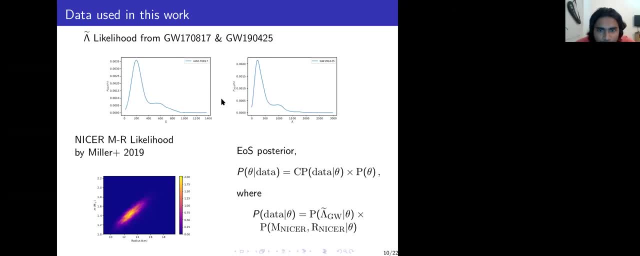 these three observations and we'll put a joint constraint on the Newton star equation, And that way it can be done through a statistics called Bayesian statistics. So I think most of you do not know about the Bayesian statistics in that much, So I'll go through it a little bit slowly. 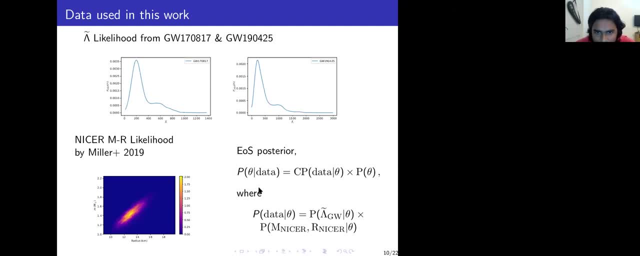 So this equation is called the Bayes' Theorem actually. So the left hand side of this equation is known as posterior. so which is the probability of getting the equation set parameters, which is the theta, in this case even the data. So in our case the data is these three data. So this is the 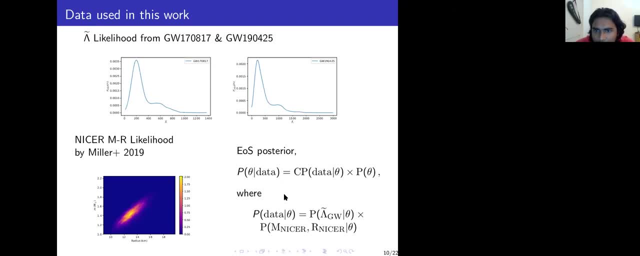 quantity we are interested to calculate Now. this, equal to some normalization. constant c- let's forget about that right now- times this probability, which is known as likelihood, And this probability is that: what is the probability of getting the data given? equation of set parameters. 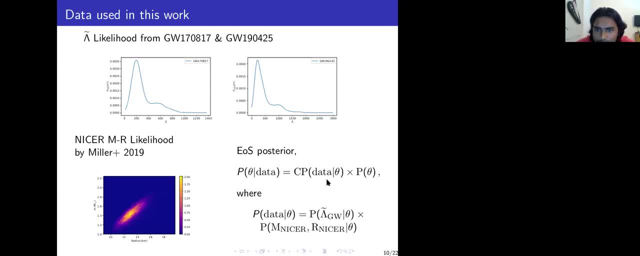 So let me explain: how do one calculate this probability. So let's say we are right now interested in GW17Z17 data only And for some equation of set parameters we have calculated this quantity, lambda tilde, to be 1000.. So now, from this plot, 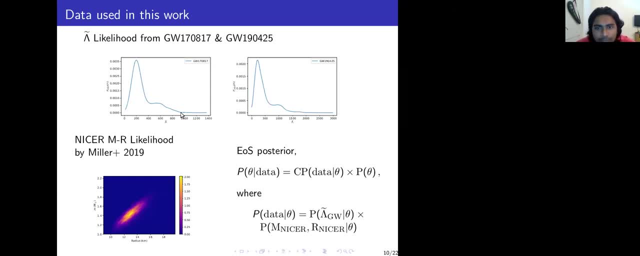 you can calculate that probability is very low. And for some other equation of set parameter, we calculate this value of lambda tilde to be around 200. And that probability will be very high, So that parameters will be more likely compared to this parameter. 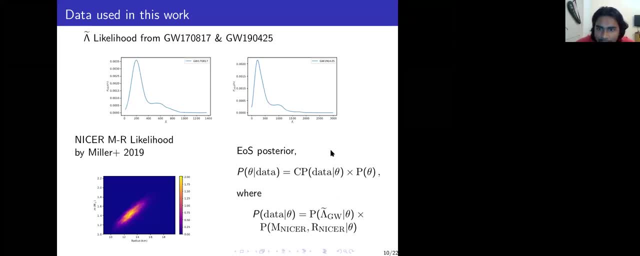 So this is that information actually contained in this likelihood, in this likelihood- And P theta is called a priors for each parameter, which I have already discussed in my previous slides. Now, in our case, the likelihood will be combined and the likelihood 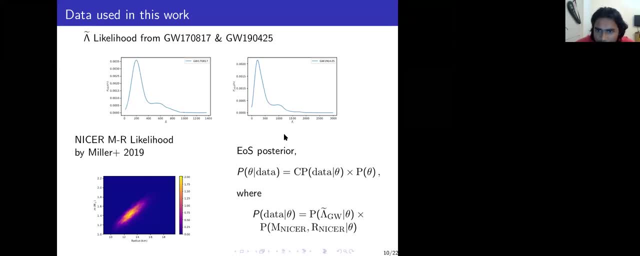 So the combined means these three observations will be combined. So since these three observations are independent observations, so the probability we are getting from this observation can be multiplied so, which is shown by this equation. Now, the computation of this equation is very expensive. 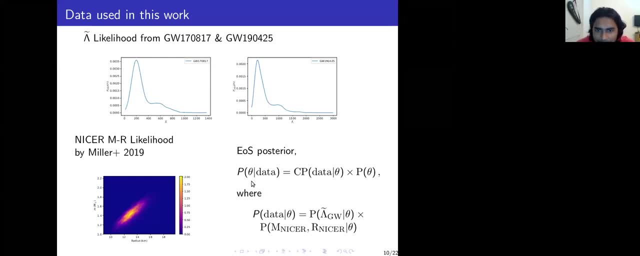 So imagine so you have six parameters, equation of set parameters, And you want to compute this quantity So you can proceed with some grids, right? So for each parameter you can choose 10 grid points. Then the number of operation you have to do is 10 to the power six. 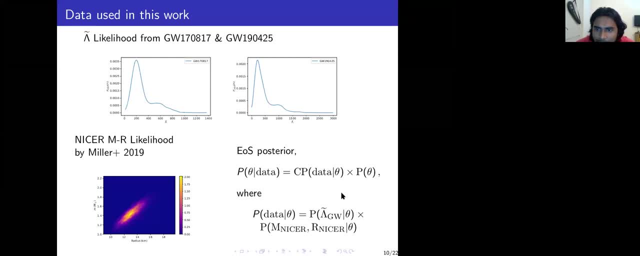 And that operation is actually time consuming And you're not sure whether the 10 grid points is enough or not. You may need to choose many grid points. So to tackle this problem, one choose various type of sampling algorithm, And those are called. 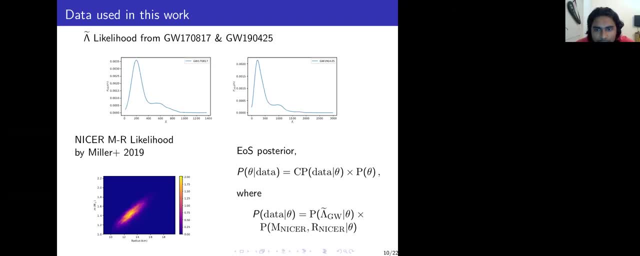 Markov chain. Monte Carlo sampling algorithm. There are nested sampling algorithm also, So unfortunately I do not have time to go through about those sampling algorithm in this talk. But just keep in mind that using those sampling algorithm one can compute this equation. 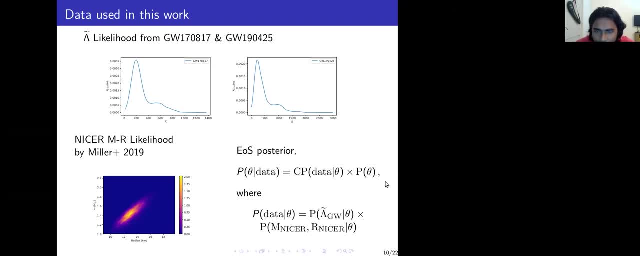 which is much more easy for the computation time. Now this thing is computed, you know, in our paper, using the population facility which is available in Ayuka, So the Pegasus cluster we used for this computation And we use a nested sampling algorithm in our calculation. 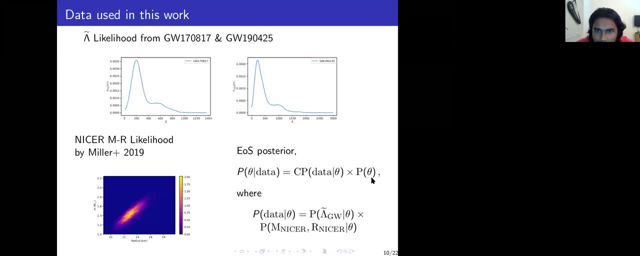 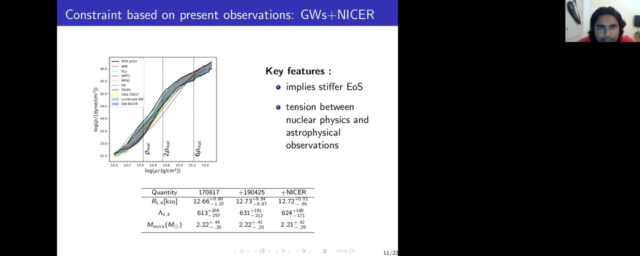 So which are now available in various Python packages also. Now let's talk about the results. So here in this slide I'll be talking about the constant which we are getting from the current observations. That means combining these two, combining GW and NYSA. So here this plot is the equation of state plot. This is plotted: 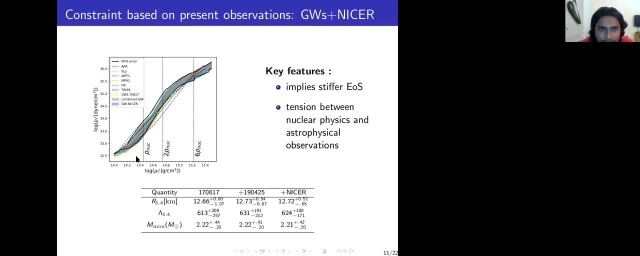 in a log scale, The o-axis is the pressure and the x-axis is the energy density. So the yellow one is the yellow band is coming from the GW 17 08 17 data atom and the green band is coming when we are combining GW 17 08 17 and GW 19 04 25.. And the blue one is: 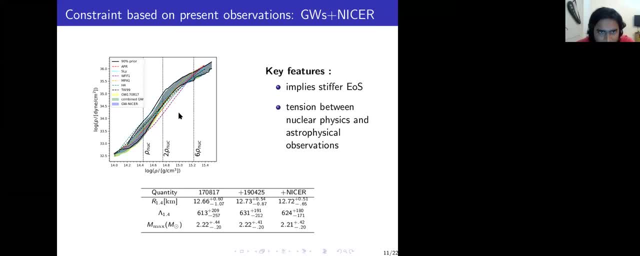 coming from the GW, both GW and NYSA. So from the plot it is very difficult to distinguish between this yellow and green, because the second GW observation was not allowed one. So it does not help that much to constrain the equation of state. But when we add the 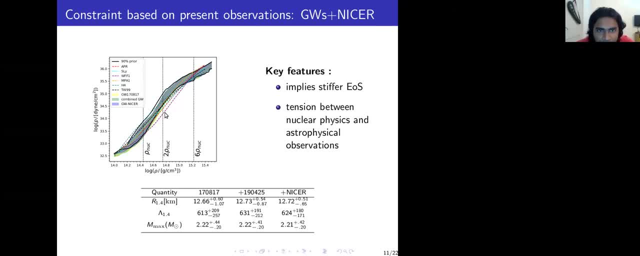 NYSA data, we get little bit constrain in the equation of state plane. Now the interesting thing which are observed in the equation of state plane is that the equation of state plane which we are observing in our study, that this astrophysical observation imply. 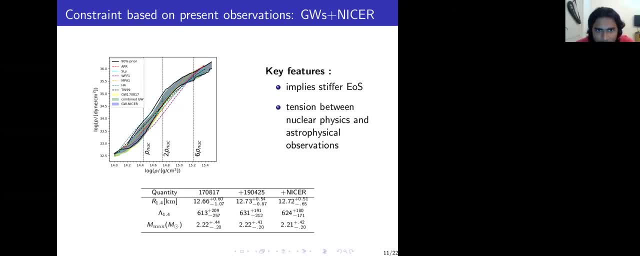 a little bit stiffer equation of state of the neutron star compared to some previous studies. So there are some previous studies which has been done using some different equation of state parameterization done by, for example, it has been done by LIGO-VALGO progression. 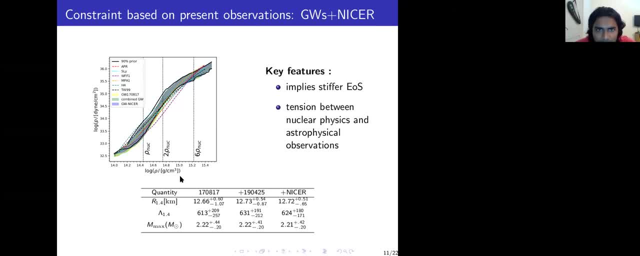 also, And they found the equation of state of neutron star to be little bit softer. So, for example, here we are getting this value, lambda 1.4, which is tidal deformability of 1.4 solar mass. neutron star around 600. with some error burn, But they found it around. 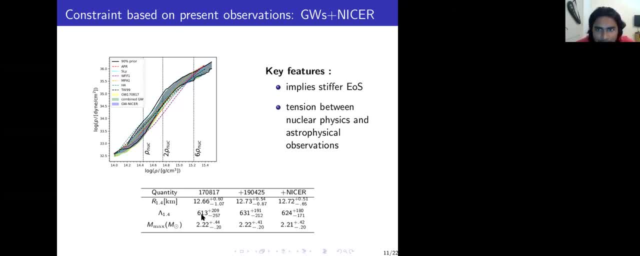 300 with some error burn. So now we can see that we are getting stiffer equation of state posture. So the reason is that our nuclear physics model is nuclear physics is informed by the nuclear physics, But they chose some equation of state parameterization which 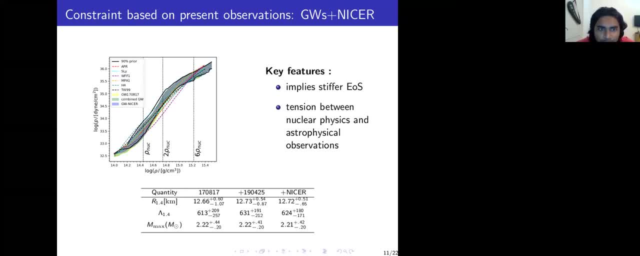 are not available in the original model. So this is the lag of the equation of state, a kind of agnostic to nuclear physics. So we are finding a tension here between nuclear physics and astrophysical observations, and the conclusion is that it is very difficult. 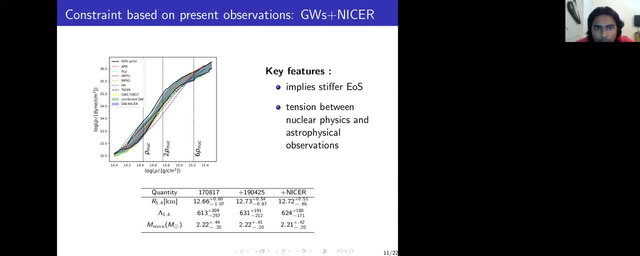 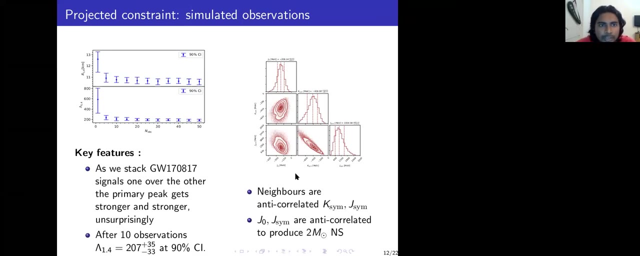 for nuclear physics to reproduce the softness in equation of state, which actually demands- which the astrophysical observation demands- keeping the two Salamas constant. Now let's talk about how the projected constant will be. So, here in this study, what we have done, 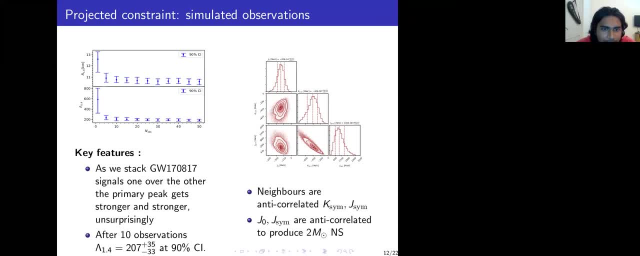 we have stacked GW17Z17 light signals one after other and we show here the evolution of R1.4 and the lambda 1.4 as a number of observations. So you can see, after 5 to 10 observations the median value of this quantity shifts from a higher value to lower value. So that is because 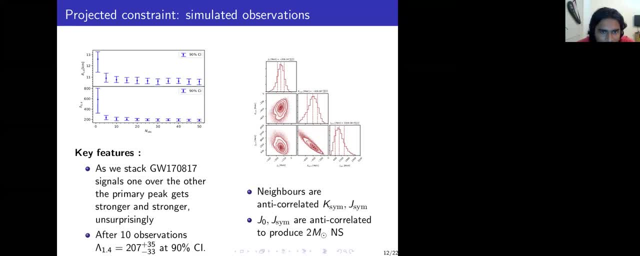 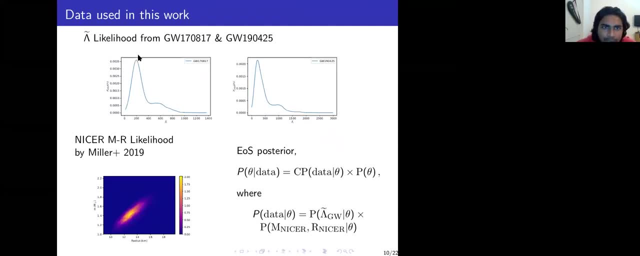 as we are stacking GW17Z17 light solution one after another. So if we go back to this lambda tilde likelihood here, if we stack this type of signal one after another, the contribution coming from the primary peaks will be more, higher and higher, And after 5 to 10 observations, 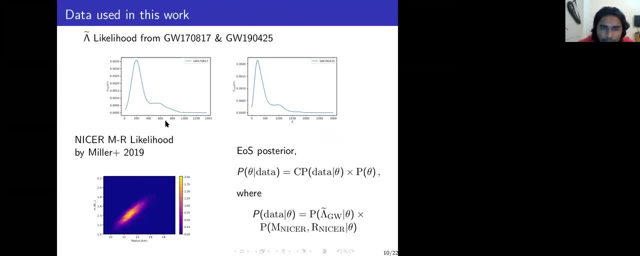 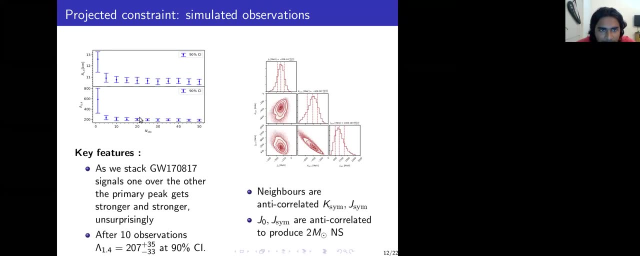 the contribution coming from this peak will be very lower. So now that's why the contribution will be coming from the primary peak only and these values are getting shifted to a very low value of radius and lambda value of radius, low value of lambda tilde. So after 10 observations, 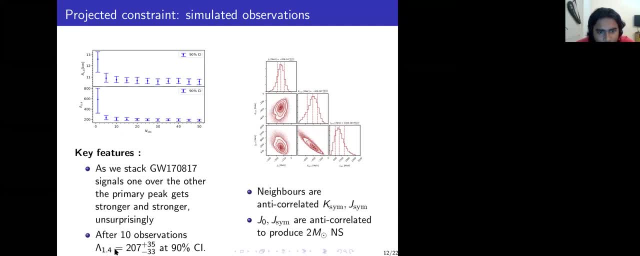 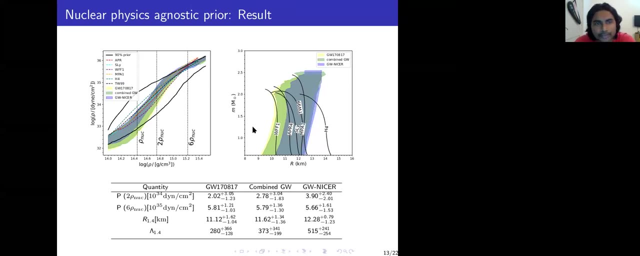 the value of lambda 1.4 will be 207 plus 35 minus 33.. So, okay, I think I am running out of time, So for the time being, let's not discuss this plot. So in our study we have demanded that. 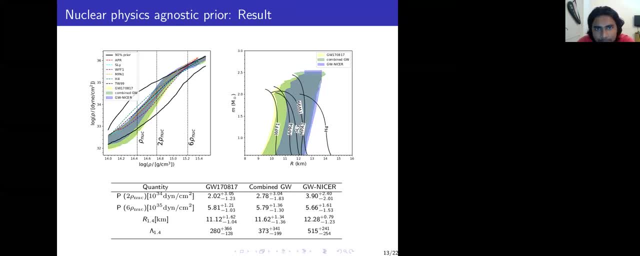 there is a tension between nuclear physics and astrophysical observation And we believe that that tension is because of the, because our nuclear physics parameter is informed by the nuclear physics experimental results. So remember, you know, when we choose the prior for our nuclear physics parameter. 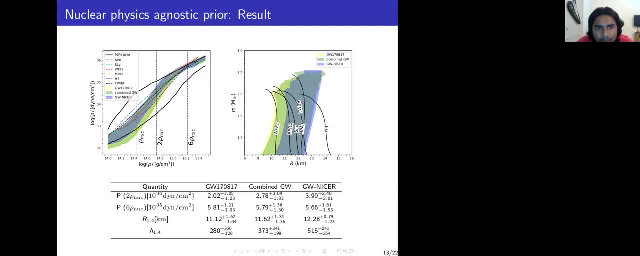 we kept fixed few of the parameters and also we chose Gaussian priors for a few of the parameters. So now if we, instead of doing that, if we chose a broad prior for those parameters, then our parameterization will also be agnostic to nuclear physics And choosing that kind of prior. 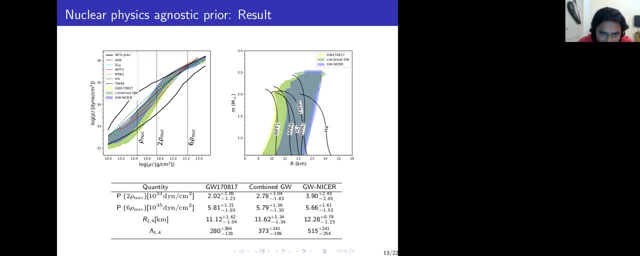 we ran the Bayesian analysis again and we find that now this parameterization also supports the softer equations set up in the system. For example, using GW17H17, we are now getting the value of lambda 1.4 around 300, with some error. 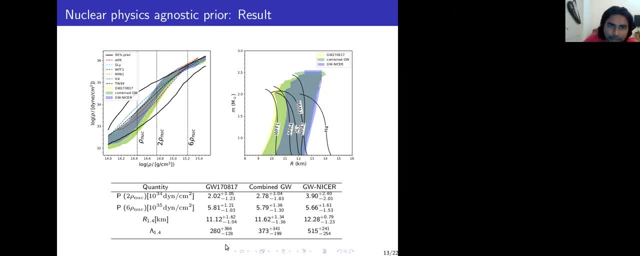 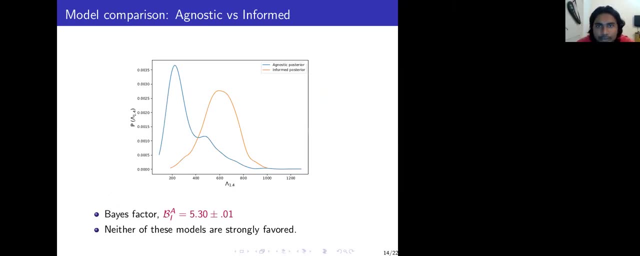 So the conclusion is that only nuclear physics agnostic model can reproduce the softness which astrophysical observation demands. Otherwise nuclear physics is in tension with astrophysical observation. Now here we do a model comparison, model comparison study between the nuclear physics agnostic prior and nuclear physics informed prior. 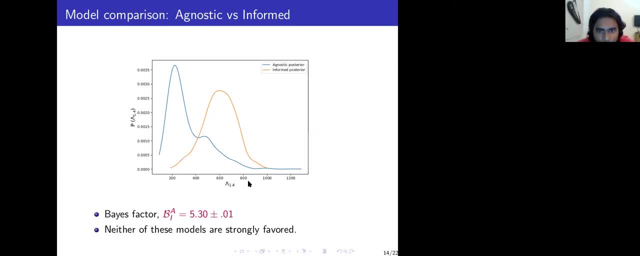 So here the distribution of lambda 1.4 is plotted for the both cases, and you can even see that the results we are getting are quite different, though there is a overlap. Now, the way one can do this model comparison, that is one have to calculate this base factor. So this is the base factor. So 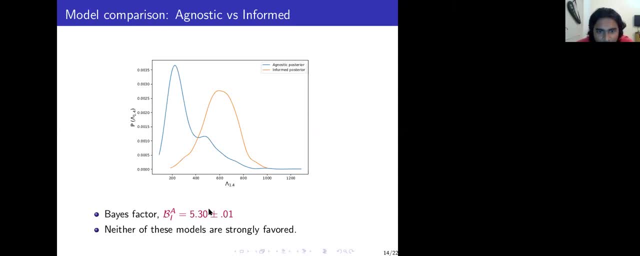 we can calculate the base factor of lambda 1.4 and lambda 1.4, and this base factor. we are getting around 5.3. And this base factor actually in favor of this agnostic model. Here 8 stands for agnostic. 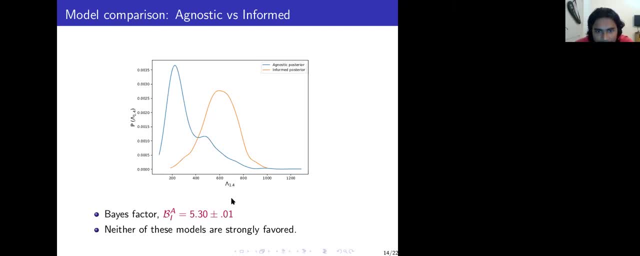 and i stands for nuclear physics informed model. So now this base factor suggests that the agnostic model actually slightly favored compared to the nuclear physics informed model. But this base factor is not that high. So that is why our paper is to be a hint of attention between nuclear physics and astrophysical observations. 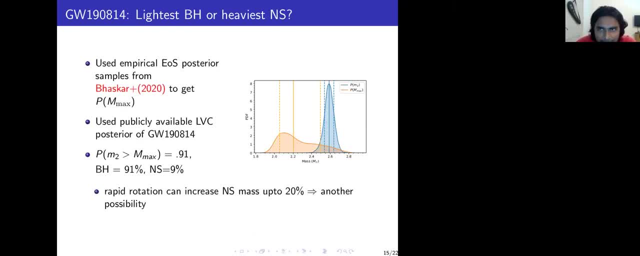 So this is where the first part of my talk ends, And I now realize I have taken a lot of time. Should I go to the second part? It's okay, please go ahead. Okay, thank you very much. So now the second part of my talk will be based on this particular GW event. 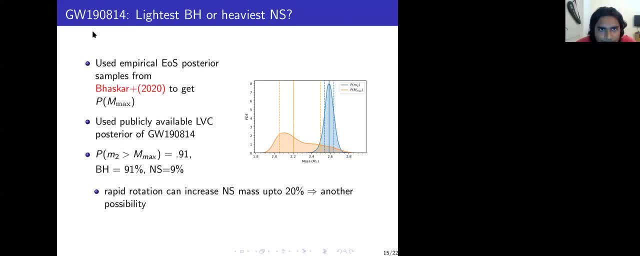 so, which is known as GW190814.. And this is the most enigmatic observation which has LIGO made so far. So this observation is associated with a 23 solar mass black hole and a 2.6 solar mass compact object. So before this observation we haven't observed any compact object which 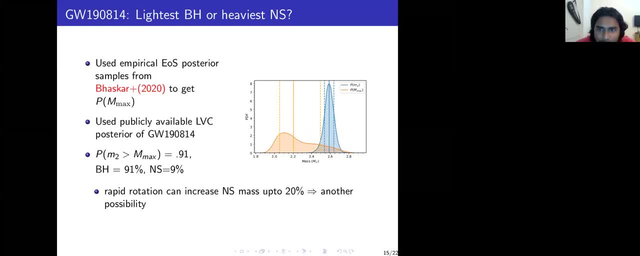 lies between two to five solar masses, Which is also known as the mass gap regime. So this observation actually gives us a unique opportunity to study the properties of this particular compact object, whether it is a black hole or a neutron star. So for this event, we didn't observe any electromagnetic counterpart. 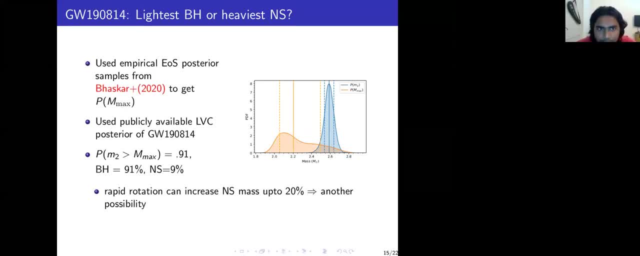 so we cannot tell whether it is a neutron star or a black hole. Also, we haven't observed any indication of the tidal deformation also. Therefore, what we have, that only the mass posterior of the secondary object, which is shown here by this blue diagram, Now in the orange here we have plotted the maximum mass distribution. 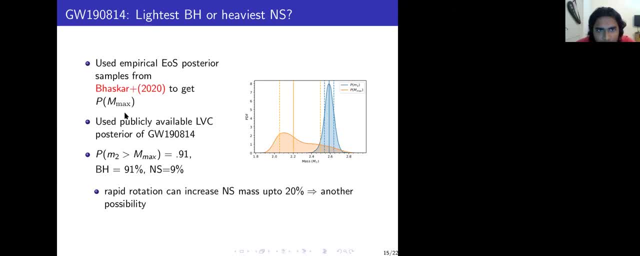 of a non-nucleotide neutron star which is obtained from our previous study. So in our previous study we used combined GW-Neusser data and concerned the equation of state of neutron star, And those equations of state are now used to calculate the maximum mass. 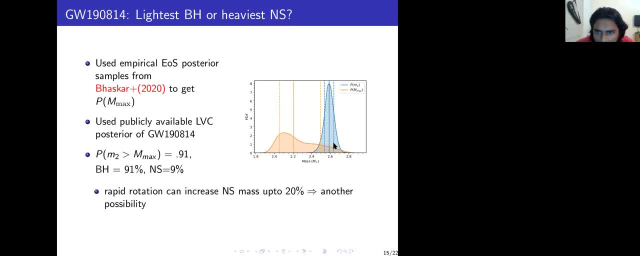 of the neutron star, And this is the distribution of the maximum mass. And from the overlap of this distribution, we find that what is the probability of this object being a neutron star? And that is, we are getting around 9%, And so the rest of the probability will be. 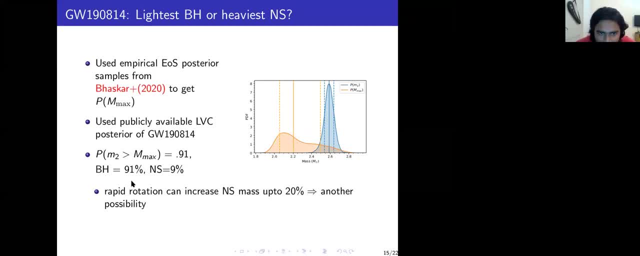 the black hole. So this is around 91%, Though we have not considered another possibility- that neutron star can also have spin And rapid rotation can increase its mass up to 20%. Therefore you can see from this graph if we allow the rapid rotation to a neutron. 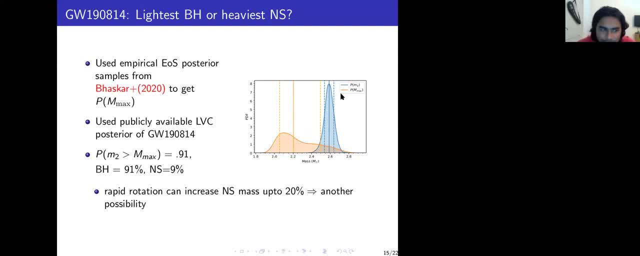 star. it can easily explain this object Now. so what we have done in this paper? we have considered both of these scenarios. One is the slowly rotating in this scenario, or non-rotating in this scenario, And another one is the rapidly rotating in the neutron. 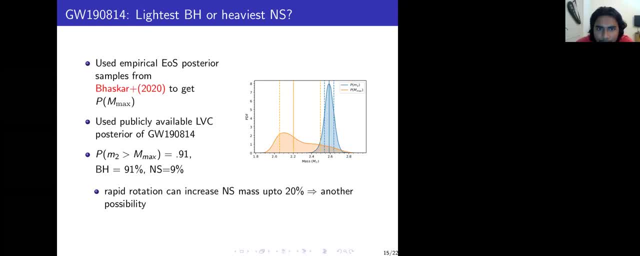 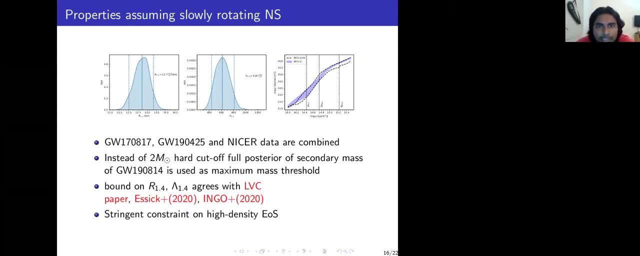 star scenario And using these both hypotheses we have constrained the properties of the properties of the neutron star, and I will be talking about that. So first let's talk about the properties assuming slowly or non-rotating neutron star. So here we used GW17017, that 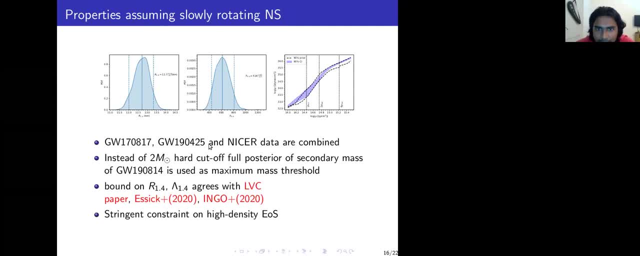 previous to GW detection and the nicer detection as a non-rotating neutron star and we combined them. and remember, in our previous paper we used a two solar mass hard cutoff for the maximum mass threshold. So instead of that here we use the full posterior of the secondary mass of GW190814. 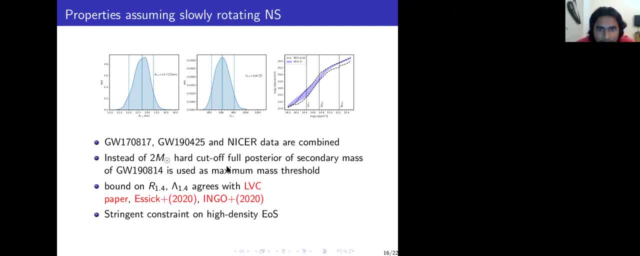 as the maximum threshold and using that we ran our Bayesian analysis again and we found this result. So here just focus on this plot that if the secondary of GW190814 is a non-rotating neutron star, it will constrain the high density part of the equation of state very much, because there are very few question. 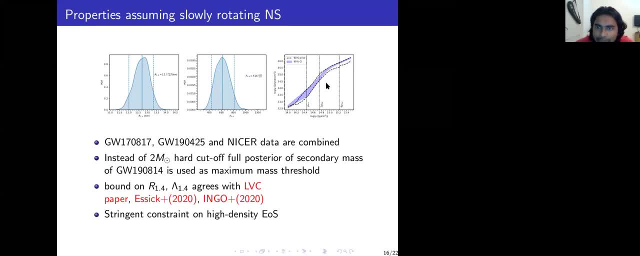 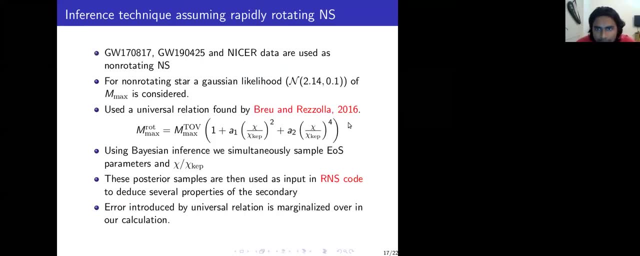 of state which can reproduce that much. so we are getting a very stringent constraint on the high density uh part of the equation. now let's move on to the rapidly locating microsoft scenario. so in this paper, for the first time actually, we have uh developed a bayesian influence technique. 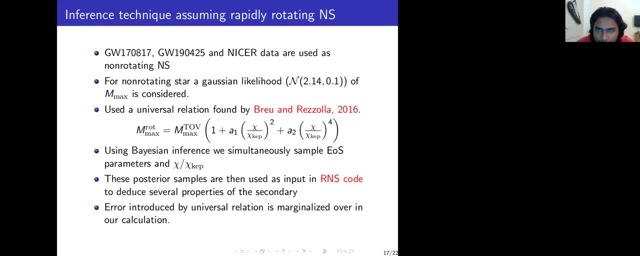 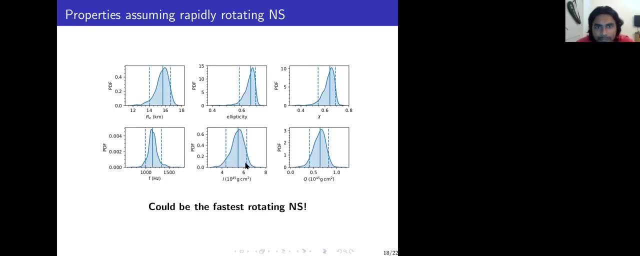 uh, to cons, assuming a neutral start to be rapidly rotating, and we have derived, we have calculated the properties of the interstellar. but, uh, since we do not have much, much time, i will not go through the details and i will go through the result directly. so here i have plotted several 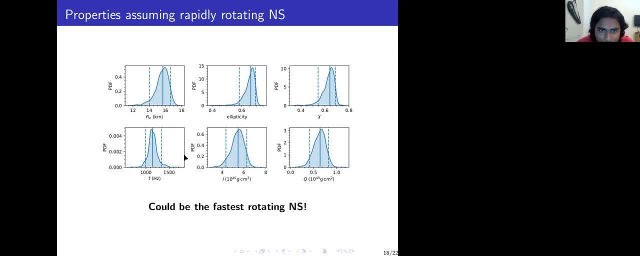 properties of the neutron star, assuming that you can study the rapidly rotating cluster. so if the nuclear cell is rapidly rotating, it will no longer remain spherical symmetry, it will become uplift, and so its equatorial radius will be different from the direction. so here in the upper left i have plotted the distribution of the equatorial 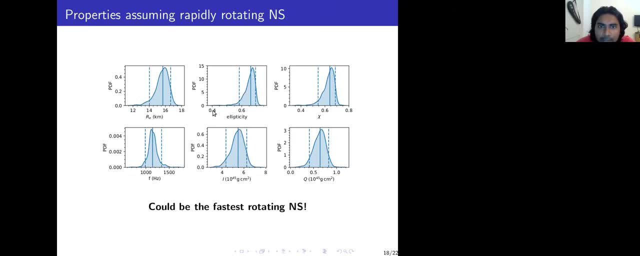 equatorial radius, and in the upper middle i have plotted the electricity of the object also. so these values are pretty high. so from this value you can understand that there will be a considerable deviation from the spherical symmetric scenario for this particular object. and in the uh bottom left i have plotted the 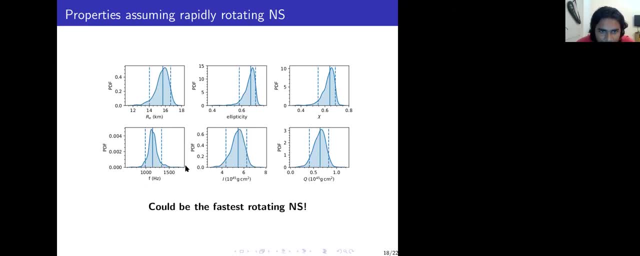 distribution of the rotational frequencies of the of the subject, and this distribution peaks around 1100 hertz. so till now we have observed the most rapidly rotating. what you observed from the radio observation is, uh, it has rotational frequency around 716 hertz. so if this object is indeed a rapidly rotating cluster, it will be the first fastest rotating. 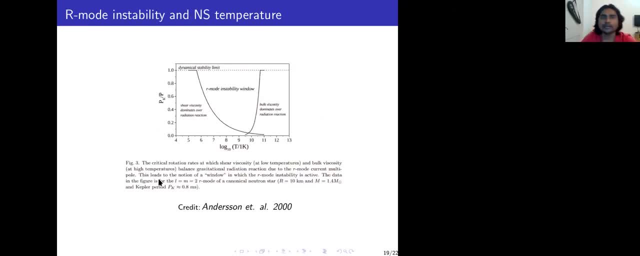 cluster observed so far now in a rotating neutron star. uh, or any rotating neutron star, are actually generically unstable through a mechanism called uh, chandra shakal friedman's roots instability. so this mechanism actually first found by chandra shakal in 1970. so he proposes that. 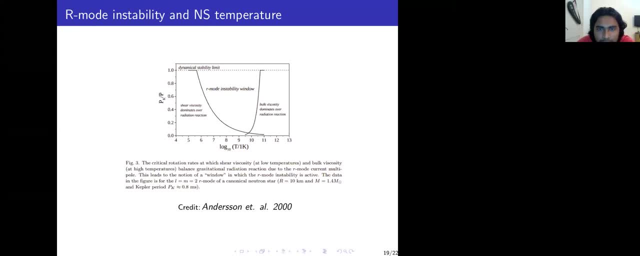 in a rotating neutron star any mode which are retrograde in a rotating frame. if they become become prograde in the inertial frame, then there will be emission of gravitational wave from the neutron star and because of the emission the spin of the neutron star will go down. 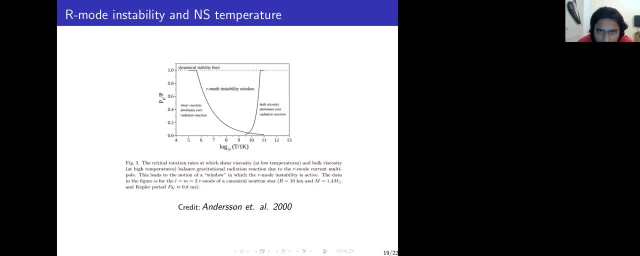 and it will eventually become a non-rotating or stochastic neutron star. So rapidly rotating neutron star cannot exist at all in nature. However, there are certain damping mechanisms inside a neutron star which can prevent this type of instability. So, for example, there is this viscosity inside a neutron star which can damp this type of. 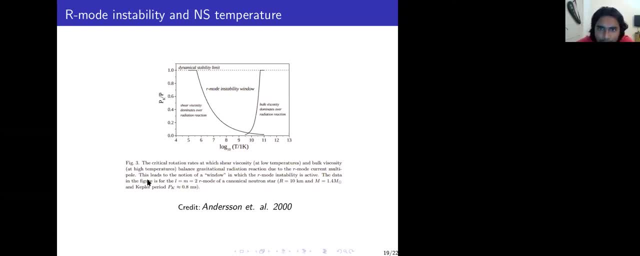 instability And this viscosity actually. so whenever the viscous time scale dominate the radiation reaction time scale, then it can actually control the R-mode instability here. So here R-mode stands for the rotation mode. So from this diagram you can see if the temperature of the neutron star is greater than neutral. 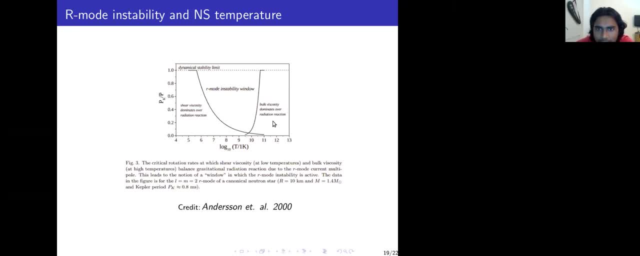 than 10 to the power 11 Kelvin, then the bulk viscosity actually dominates over the radiation reaction and the R-mode instability doesn't happen. If the temperature of the neutron star is less than 10 to the power 5 Kelvin, then the shear viscosity dominates over the radiation reaction. then also R-mode instability doesn't. 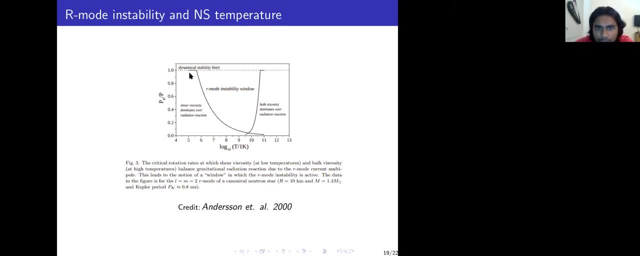 happen. But there is this window between 10 to the power 5 Kelvin to 10 to the power 11 Kelvin when R-mode instability time scale dominates over the viscous time scale and the R-mode instability happens. So now let's consider a very young neutron star which is just born and it has a very 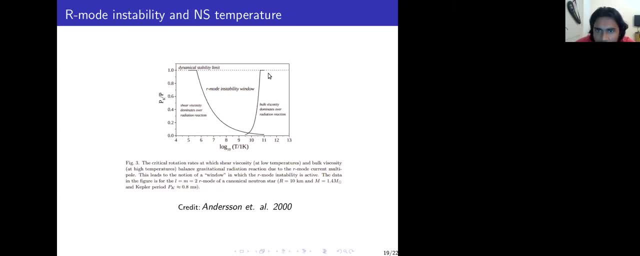 high temperature, which is around 10 to the power 11 Kelvin or 10 to the power 12 Kelvin, And it also has a very high spin. so it is somewhere around here. But as the time goes by, the neutron star will cool down and it will enter in this instability. 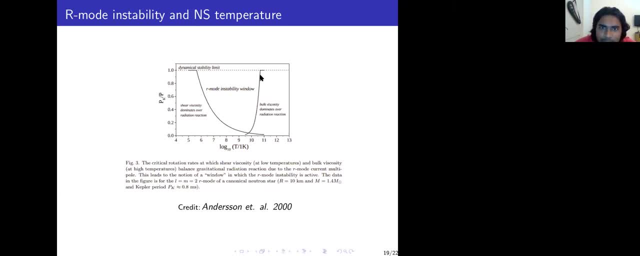 window And as it enters to the instability window, the R-mode activates And the system will emit gravitational wave from it And as a result, it will also lose its spin. So it will follow this path and it will come around somewhere here. 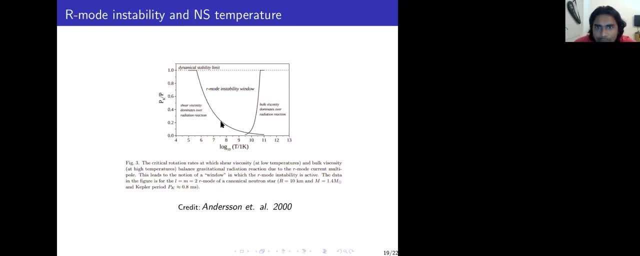 So its spin will be very down. So that's why we do not expect to observe that much highly rotating neutron star in nature. So now we are getting. if the secondary of the GW190814 is a rapidly rotating neutron star, its spin value will be around somewhere, so around 0.9 or somewhere. 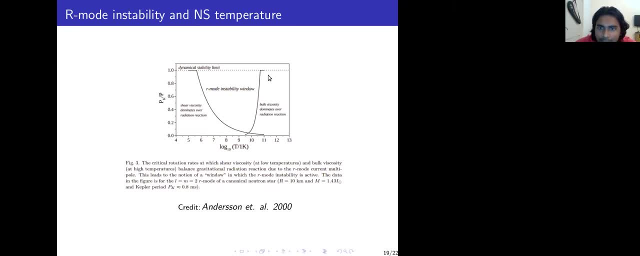 So therefore its temperature will have to be greater than 10 to the power 11 Kelvin or less than 10 to the power 5 Kelvin. Now we do not expect a neutron star to be that hot in a binary system, because the neutron star will be pretty old in a binary system. 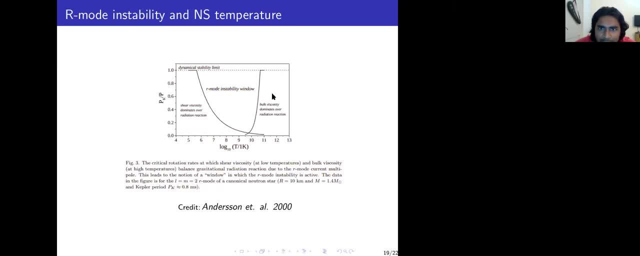 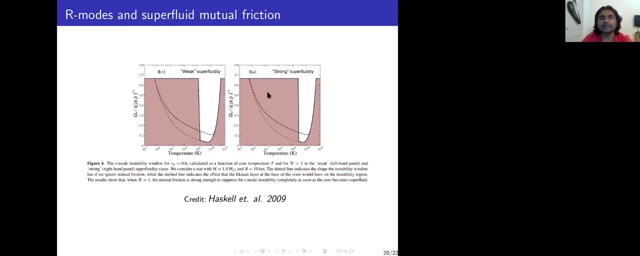 So therefore, this R-mode instability says that That type of pressure will not be that hot. That type of pressure will not be that hot. So the probability of the secondary of GW190814 being a rapidly rotating neutron star is very less. Now there are some other damping mechanism also. 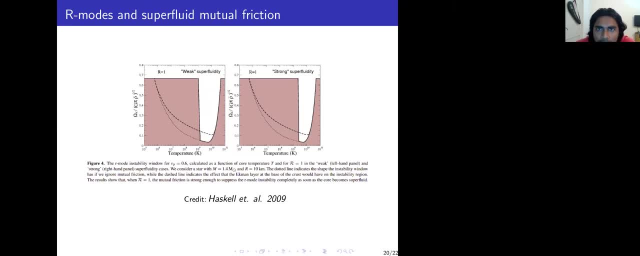 That is the superfluid mutual interaction. So inside a neutron star it is expected, it is believed, that there is superfluidity below a certain temperature. That certain temperature is around 10 to the power 9 Kelvin And below that temperature. actually the neutron star should be the material inside the neutron. 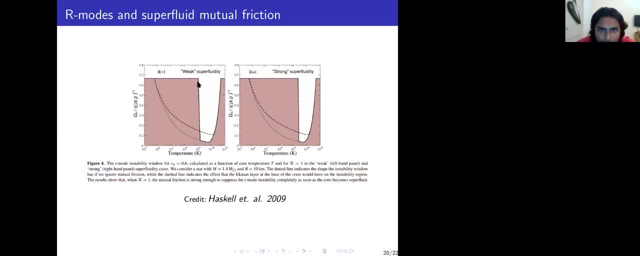 star should be in superfluid form. And if there is a superfluidity that can actually also act against this R-mode instability And, as a result, that instability in the time scale actually shrinks, So it comes around here. So now let's imagine a scenario where our secondary neutron star is a rapidly rotating. 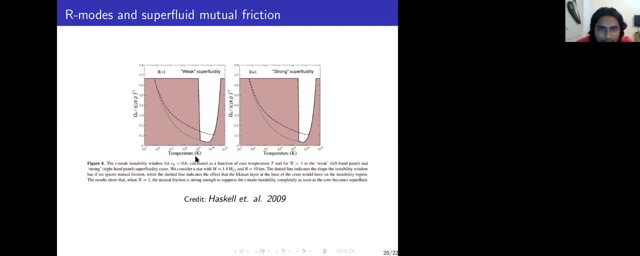 neutron star. So in this case the primary neutron star was actually initially in a low-mass還是 SABINI system and it aerates, spin from the low mass star And it becomes a very highly-pumped neutron star. Its temperature was that time around 10 to the power, 9 Kelvin. 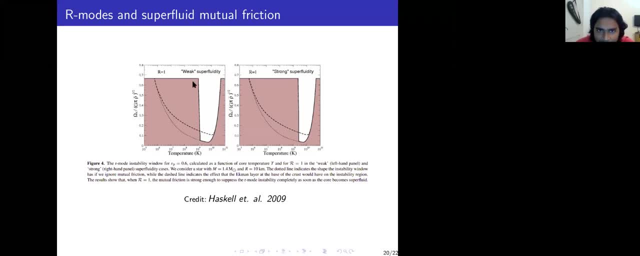 So it can stay here at that moment and that R-mode instability also will not activate for that start also. And now after that at some point it becomes a binary with that 20 Kelvin. I think that would be the answer to this. 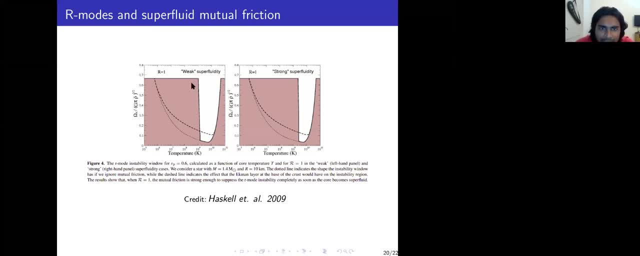 Okay, is very much black hole. So in that binary system it still can retain its spin because of the superfluidity. So in that type of particular scenario this type of system can only exist. So the conclusion is that in order to become the secondary, to be a rapidly rotating 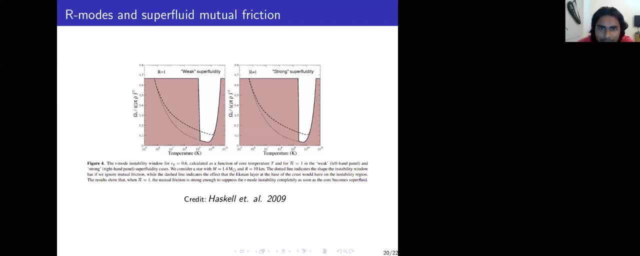 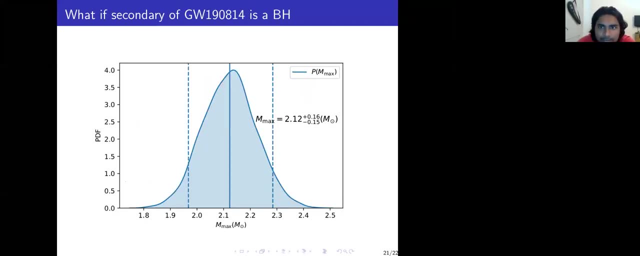 integral star. the condition has to be very extreme, Otherwise the black hole scenario is much more likely. Now the thing is, what if the secondary is a black hole, Then also it gives us a very important information about the equation of state of an integral star, because it sets an 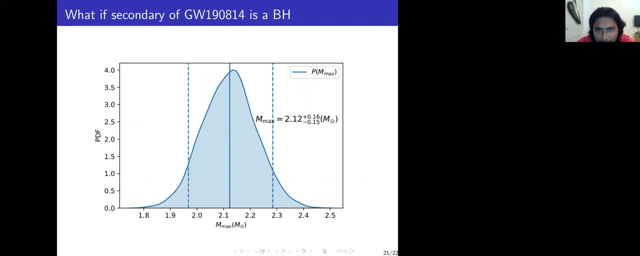 upper limit on the integral star's maximum mass And using that upper limit we have run the Bayesian calculation again and we have constrained the equation of state of an integral star And using those equation of state here we have calculated the maximum mass of the neutral star and that maximum mass distribution is actually plotted here. 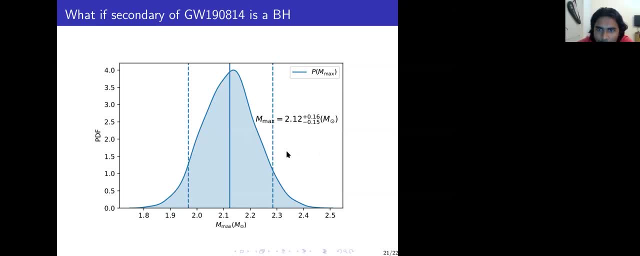 Now we are finding the maximum mass of the neutral star will be within this range. So its value will be 2.12 plus 0.16 minus 0.15.. And this is the most stringent constant which we have obtained on the neutral star's maximum mass in the study so far. So we have tested this secondary object. 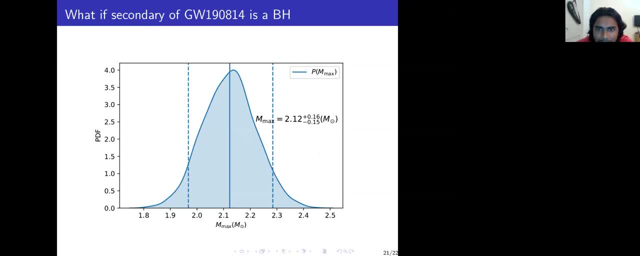 in various scenarios and each scenario actually leads to very interesting results that I have presented here. Also, if you want to know more about this object, I have also written a blog about this in LIGO in the Facebook page, So you can see that blog also. So this is the. 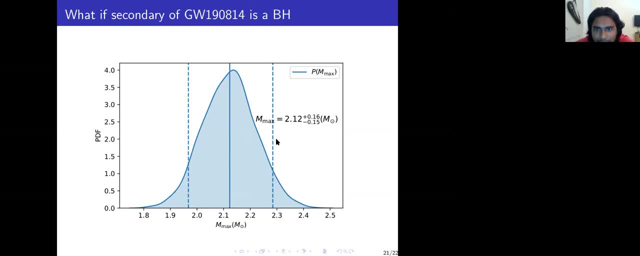 point I would like to end my talk. So thank you again very much for your patience and if there are any questions, you can ask me now. thank you so much. That was a wonderful talk. So we have a few questions. We have a question in the chat. and read that out first. 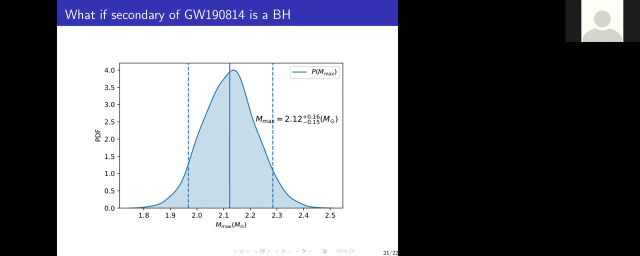 How is the ring down part of the waveform model using post-Newtonian expansion as well? No, ring down is not modeled using post-Newtonian expansion, So we use only post-Newtonian expansion in the inspirer algorithm part, so that for the ring down you use numerical relativity simulations. okay, okay, so we have a few. 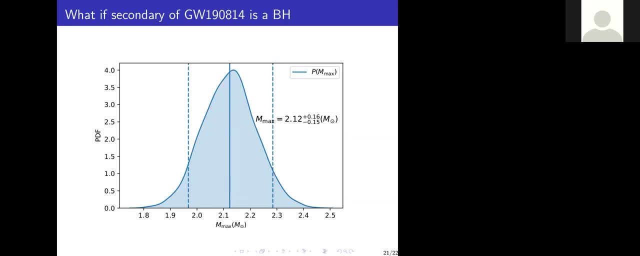 raised hands. so, shabnikda, please go ahead. um hi, thanks for the nice talk. um um, i was uh wondering that, when you were talking about the neutron star equation of state, it seemed uh that uh, the posteriors on um your like, your point was that the posteriors were very prior dependent, right. 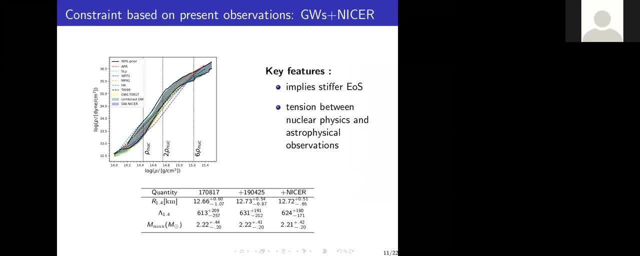 uh, like you took a agnostic model and that prior and then you had a nuclear physics informed model. you had another prior and it seemed that your posterior uh shifted a lot just because you have two different priors. now that, uh, that for to me, that me, like that, tells me that the data is not 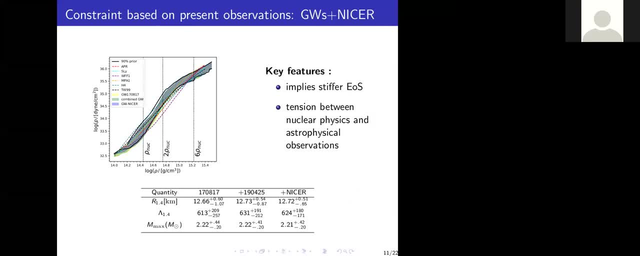 enough to overwhelm um the prior and reach a stable solution. so, like, like, do you have any kind of calculations or simulations which tells you that what are the specific or the like, the least kind of conditions or data quality? you need, uh to like, remove that strong dependence and priors and nail the difference between, like what is. 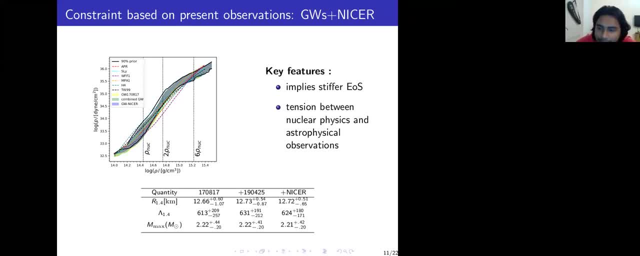 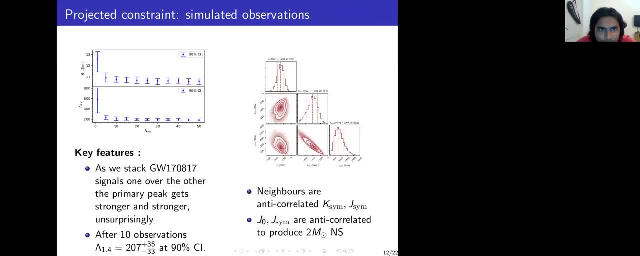 exactly going on? yeah, that's a very good question. so you're absolutely right, actually. so right now, the current data is not strong. that's why there is- we are seeing this- prior dependencies here. so if we go to this projected constant here, so when we are stacking, actually, uh, gw 17 017 like. 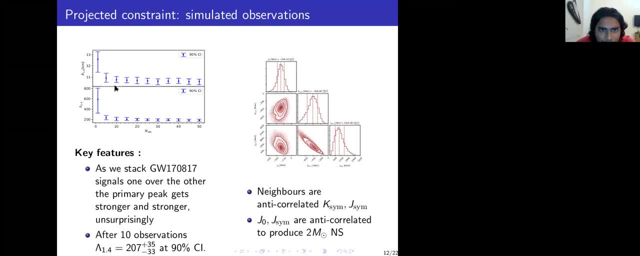 solution each on top of each other. then, uh, after five to ten observations, actually, that prior dependency will be gone. so in that case, if we use the nuclear physics, inform prior or nucleus agnostic prior, so we'll see the same results. so we have to wait for, uh, five to ten observations, uh, of same smr. 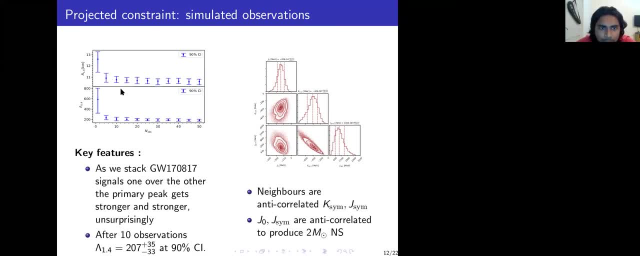 actually, uh, we can, uh we can have stronger. um, i see i had another quick little question uh, which was, uh, you were talking about rotation and obliqueness, uh, in neutron stars and uh, like when i work with exoplanets, there is this uh idea that uh, rotating exoplanets produced uh more. 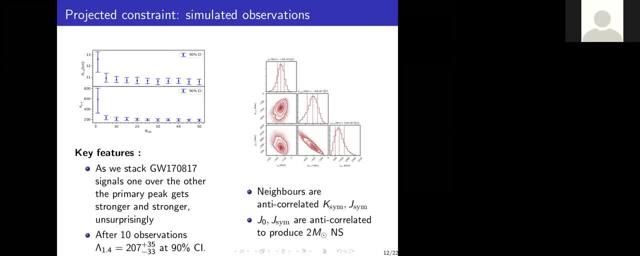 polarized signals uh than uh non-rotating exoplanets. so does, like polarization study in neutron stars or like something like that, help you in constraining that, so constraining exactly which property uh, constraining the rotation of uh, the neutron star, like you are trying to see if the neutron star is. 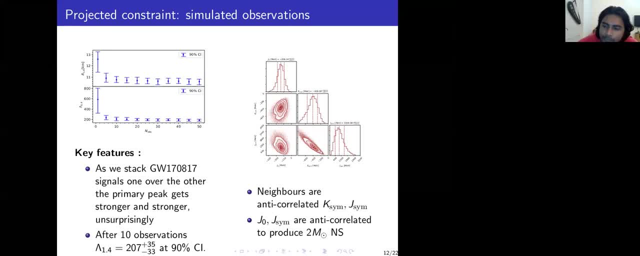 highly rotating, right? yeah, so the way it has been approached it is completely a- uh, generalistic calculation. here we are doing so. uh, for the rotating neutral star, here we are using the three plus one adm calculation and that is pretty robust. actually, i do not see how the progression actually helps to constrain the. 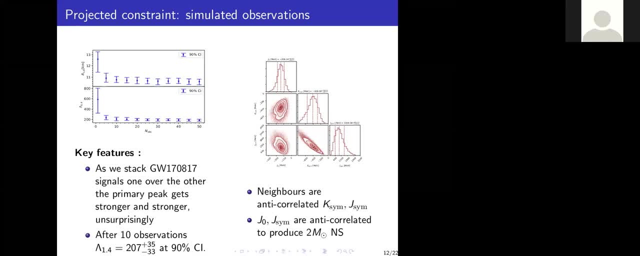 rotational frequencies. uh, so i am not talking a lot like if you have a rotating body and it's perfect, so these are all, um, like, these are our point sources, right? so if you have a rotating uh body and it's completely symmetrical, uh, sorry, non-rotating body, it's completely spherical. 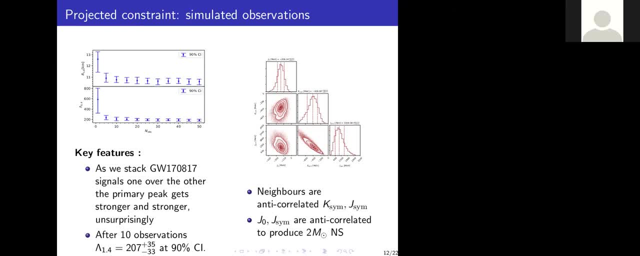 these are not point sources here. i am talking about, like electromagnetic observations. um, when you follow these up with electromagnetic observations, if you have a point source, then, um, the polarization signals tend to cancel out. but if you have an obliqueness, the disintegrated correlation signals are enhanced. 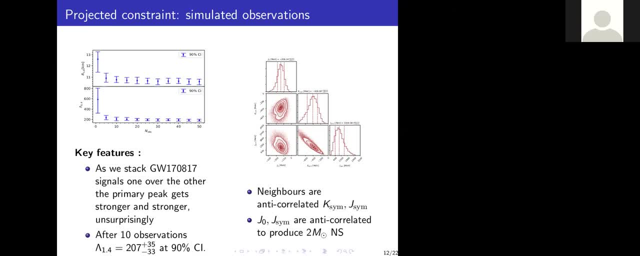 so i am talking about those kind of observations, like if you think those will happen, but yeah, that's fine, we can talk about this. yeah, i think so. um, okay, so, rc sir, please go ahead. hi, bhaskar, can you hear me? yeah, i can hear you. okay, very clear talk. thank you, uh, i just had uh. 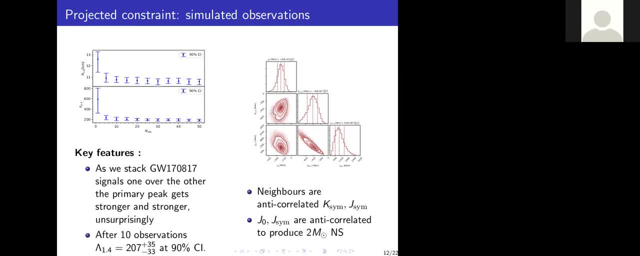 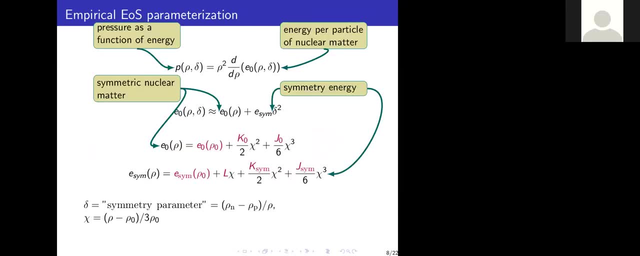 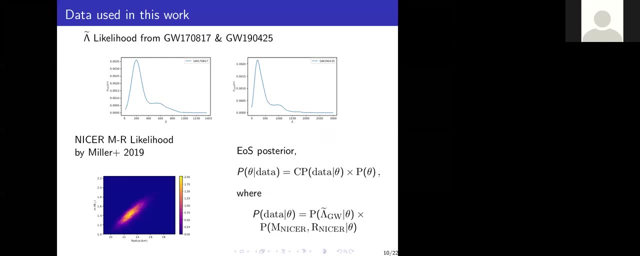 actually i have a couple of questions. so one is: when you showed the parameters of the neutron stars in those three cases, the, the 2017 neutron stars in those three cases, the, the 2017 neutron stars in those three cases, the, the 2017, the, the two gw and one nicer result, so those parameters seemed i mean. can you go to that? 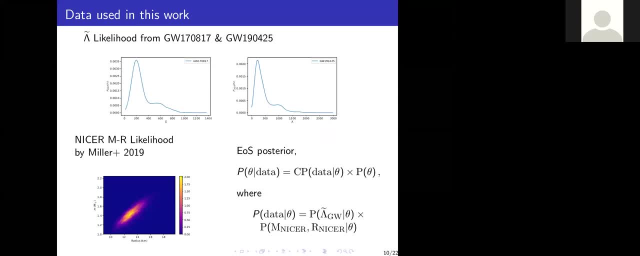 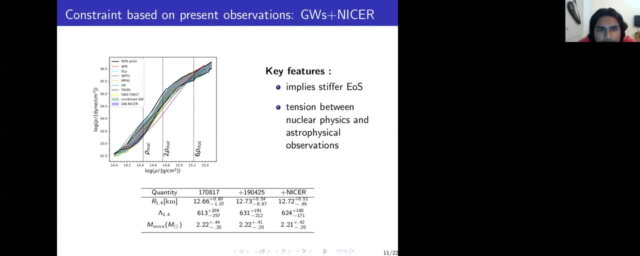 slide that, uh, i think, then the slide, no, i think, the next slide or the next slide, yeah, this one, these, these parameters, these are lambda and max. they seem extremely, you know, close to each other. i mean, is there any reason why all all these cases have, i mean, you know, neutron stars still have some? 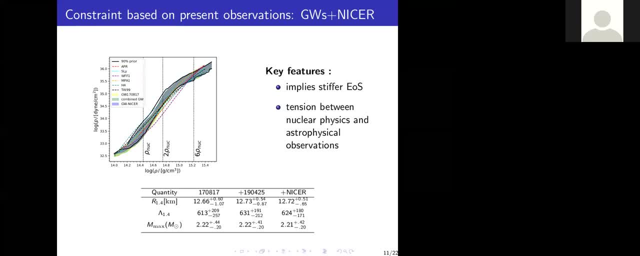 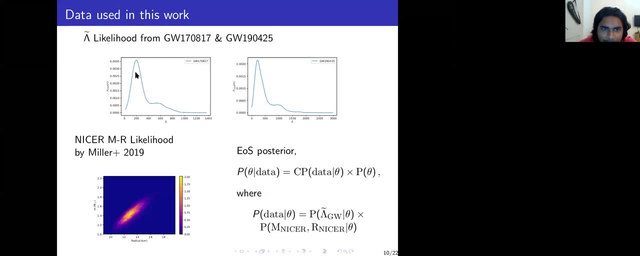 you know, somewhere i change parameters, right, why are they so close? yeah, so that is happening because of our prior choices, only here. so if you see here this laminar likelihood, we're not choosing, uh, the nuclear physics informed triode they instead of uh, preferring this peak they are. 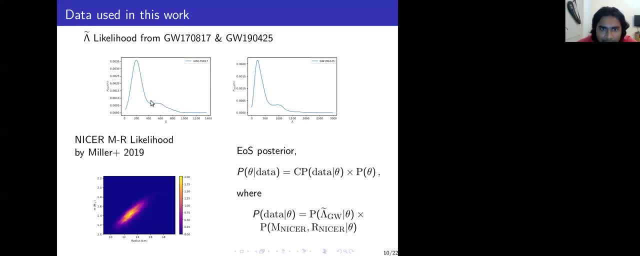 preferring actually that peak, okay, and and so. so we're getting a steeper equation for posterior because of that. uh, second is that this particular observation is going to be a little bit more, uh, this particular observation that doesn't add so much information, because this observation is: 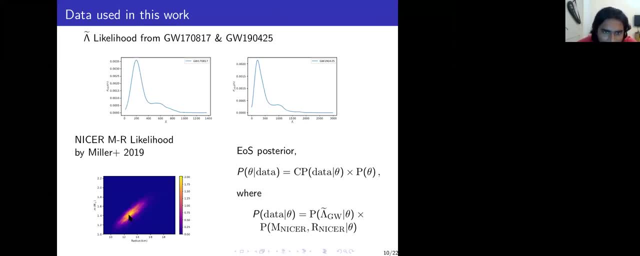 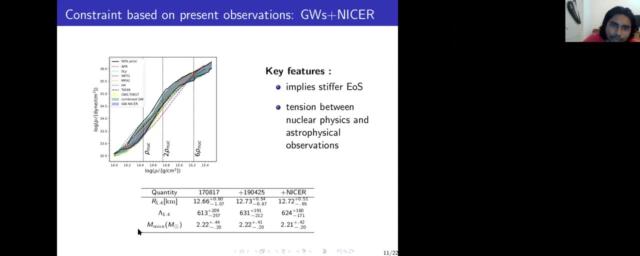 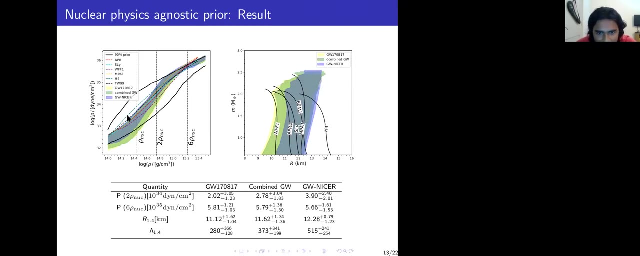 very noisy. and third is that coincidentally- uh, this nicer observation- they also particularly favor stiff equation of set, so these two actually coincides because of that. but when we're using actually agnostic prior. so in that case, uh, gw 17 017 actually prefers the primary peak. 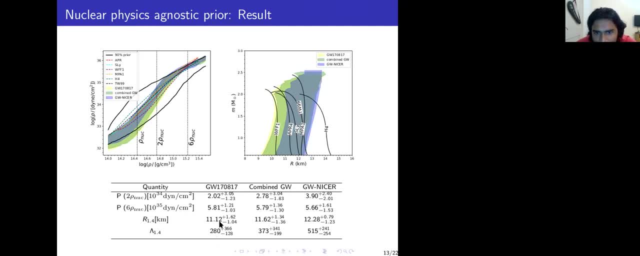 so in that case you can see, uh, that, uh, this value are quite different, a little bit different, uh, in compared to when we are adding nicer. so that time we see the difference. so it's because of the priors. okay, i'll, i'll let other people ask questions. all right, uh, assistant, please go ahead. 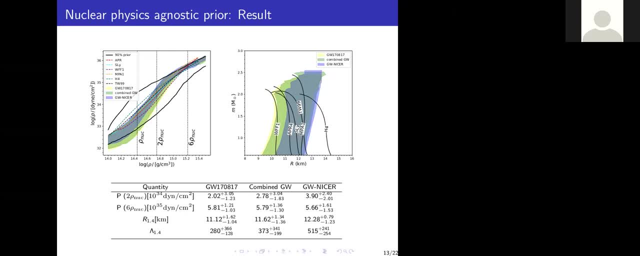 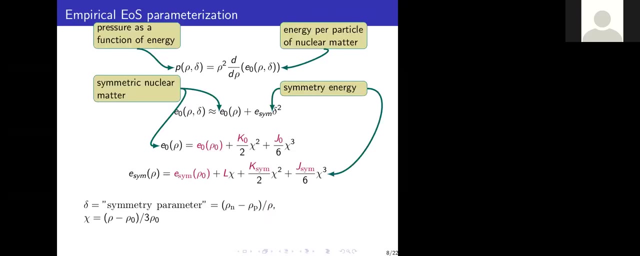 well, first of all, that's a nice talk. so again, i have also a couple of questions, must i'll ask the first one of them only so you started with the parameter using by the taylor expansion correct, where you have uh four, four parameters, uh six, but yeah, four parameters, i think, if i remember correctly, or six uh six, i mean it depends. 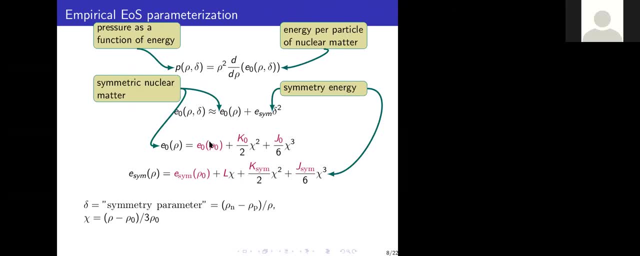 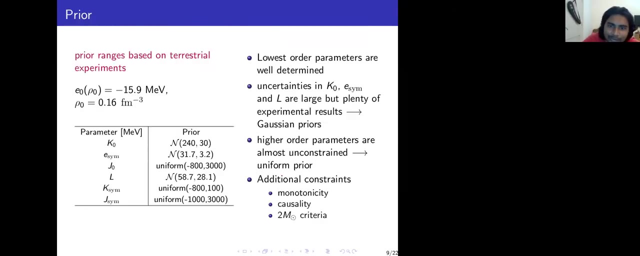 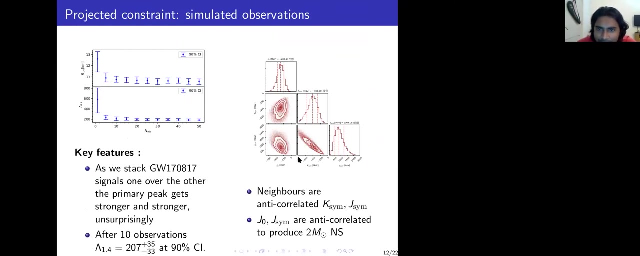 so here, eight parameters are there. so we take two parameters. yeah, so, but uh, ultimately, when you are discussing, you are showing only the likelihood of the lambda, what happens to the other parameters. so i have, i haven't shown any figures, uh, of this parameter. so i here, i had one figure which contains only three. so, uh, this figure. there there is this, this. 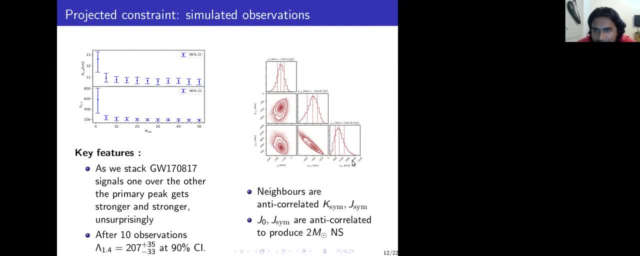 is the con uh corner plot between j, zero, k, sim and jc and there there will be also the other parameters in the l and k naught. so those parameters are marginalized over. so i haven't shown those, those plots here. so those uh parameters are marginalized over when you are doing the lambda. 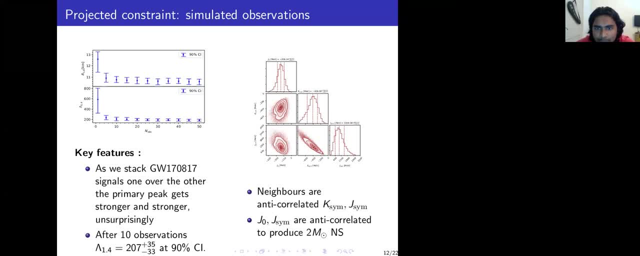 correct? no, so now what we do? now we have constant these parameters. now, using those parameters, we run again our uh pov. i mean that we again solve the general literacy equation and calculate the mass radius lambda and that, and using that, we actually plot this kind of posterior. sorry so you. 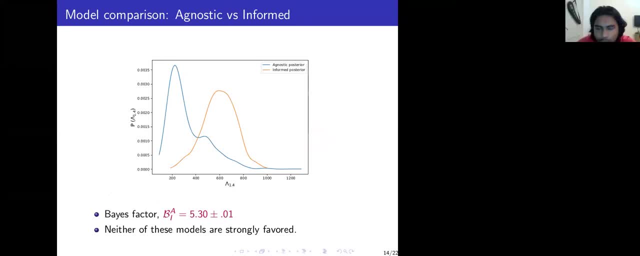 fix those values at the maximum. no, no, no, we didn't fix those values. we take all those parameters, yes, and now, taking all those parameters, we again calculate, uh, the mass radius and lambda, and that lambda and that that is plotted here and that gives us this distribution. this is distribution. 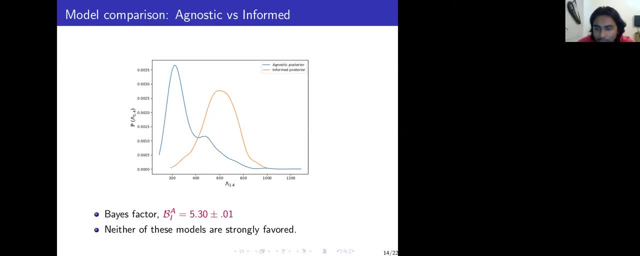 for lambda only, not the person. so the thing is that when you have the equation of set parameter, using that parameters you can plot any distribution. okay, by running the pov equation again and also the solving the lambda again. so this is kind of basically marginalized over the other parameter you are saying. 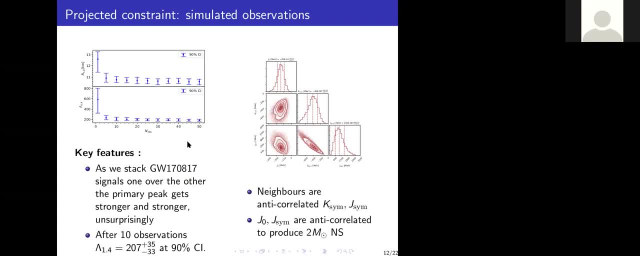 in a different way or not. i'm getting it wrong. so my question is what the other parameters means? which parameters are coming out in this plot, here? this one distribution? this is, i understand. this is uh. with some of the other, yeah, but when you are talking about the 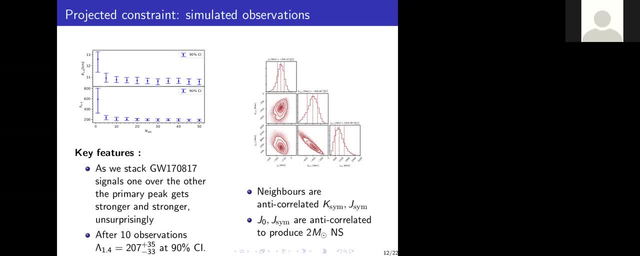 lambda. one parameter, that person, that distribution, that is marginalized. so what the equations? but they are interlinked, isn't it to related to the mass and the radius? yes, they are not independent of each other, yes, so how can you just make marginalize like that and find out the mass relation from the only one parameter? 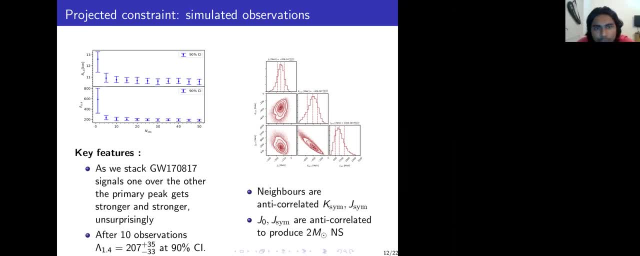 no, no, no. so from the observation and the quantity which are actually considering, those are the equations, set parameters, right now, given equation of split parameters, we again can find out what is the mass and radius and lambda of interest. so now from the, let's say from the observation- we have constant regression parameters and we have 100 samples of it. 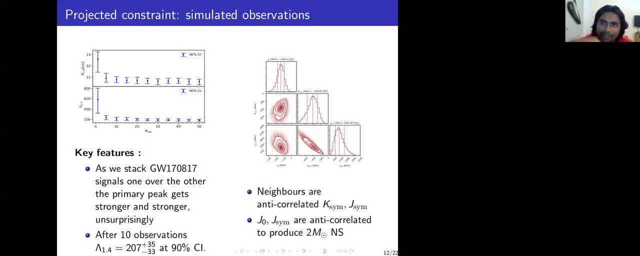 so using those 100 samples, we have calculated the mass radius lambda each times and that distribution actually i have, i'm showing in this plot. okay, fine, uh, uh, i look for you. you're still confused. yeah, it's fine. okay, uh, all right, we have a question. in the chat from ohio, she has uh agnostic and informed model for. 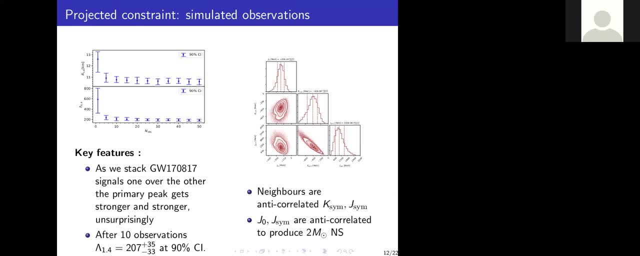 why is the middle profile is intersecting at a point? does that point have any significant? uh, sorry, your voice is breaking. i couldn't hear the last part. oh sorry, sorry, i'll dip it. yes, um, you can hear me now, right? yes, i can hear you. okay, she says agnostic and informed model profile is intersecting at a point. does that point have any? 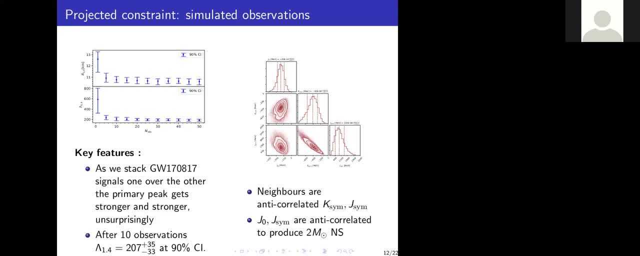 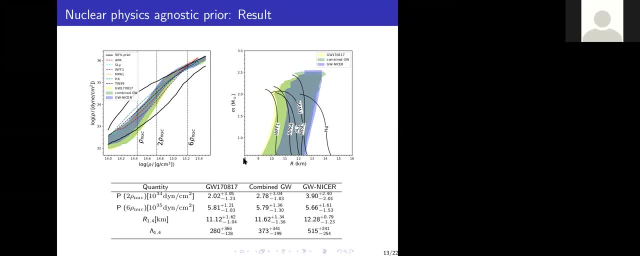 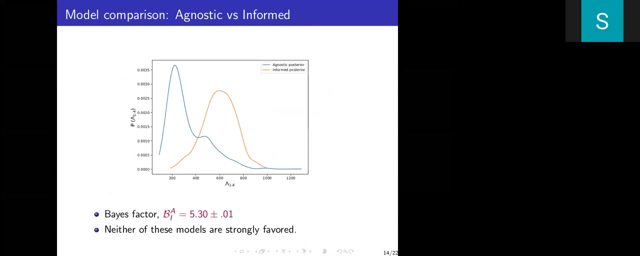 significance. uh, at which point point they are intersecting. so can you unmute yourself? can you go to the slide first car? maybe that is going to help. I think I'm so. that's like right agnostic trial. I thought there was some other distribution, that's like. so there is. 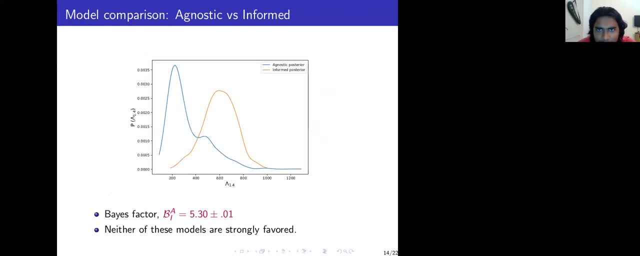 interesting intersection, right? so yeah, yeah, that this one, yeah much got that. yeah, so it is not that that they are completely giving a completely different results, so they have some intersection. that's why, when you are studying this model comparison, we are not getting very strong significance here. so this base 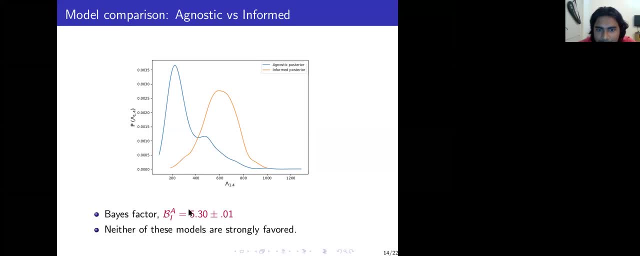 factor is giving a. I don't giving us a very, very weak had- actually not very weak, but it is a substantial value, of course. so we cannot actually distinguish between these two models from the data. so, if I can just make a comment, we know that that's. 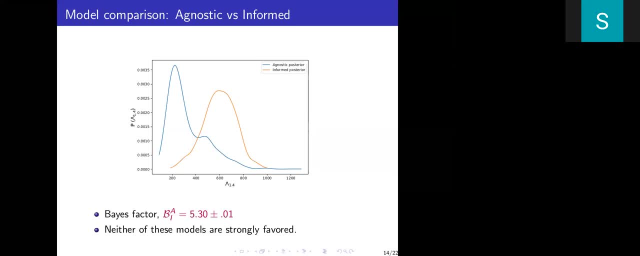 actually the PDF, the probability distribution. okay, so that's not the model profile or anything, that's the probability distribution of what you get of that lambda parameter. think so, ma'am, please go back. okay, thank you, Bhaskar for giving the talk and also good talk. I just have him, I think, a very basic question. so my question is: here we have this: 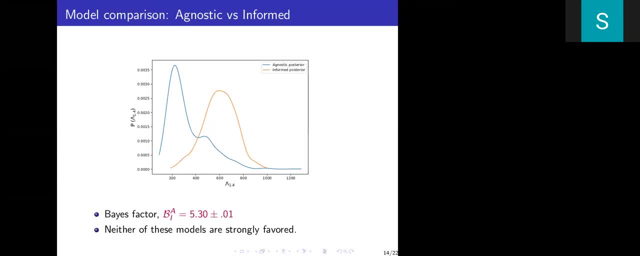 three, four, five, three. I think you mentioned three four, five and you know, I think I am thinking of this question and I am thinking of the next. I mean, maybe I want to go back to the last question. I am already, but I'm looking for another one, but I don't know if. 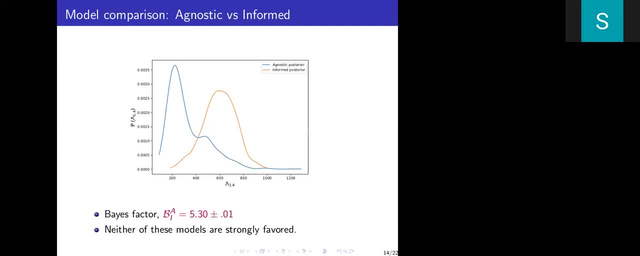 you want to do it right now, or I think I don't know if I need to like fix it on this one. two GW observations And we have these equations of state models from nuclear physics input. Now, as far as so, two data points, I don't is not a big data set. Also, my concern is that 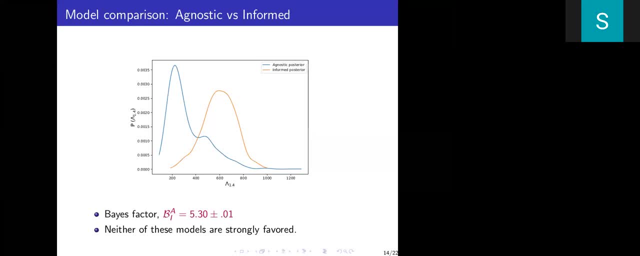 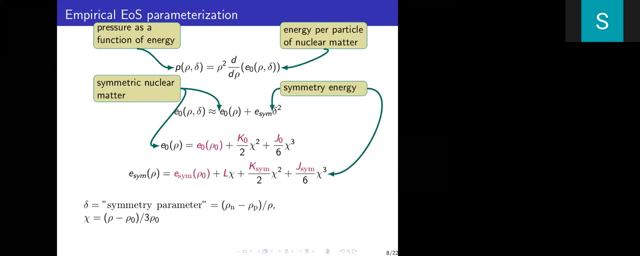 how robust are those nuclear physics predictions of models? I mean, when we are saying that we are constraining equation of state? how good are our understanding of the theory itself? Can you comment on that, Because neither there are a lot of data nor I don't know. I mean 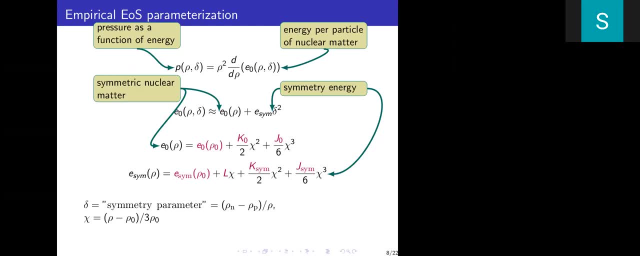 how robust is. are these all nuclear physics things? or you have QCD involved here. So we didn't consider any microscopy interaction here, We just more model it from based on the saturation properties here. So what we have done that 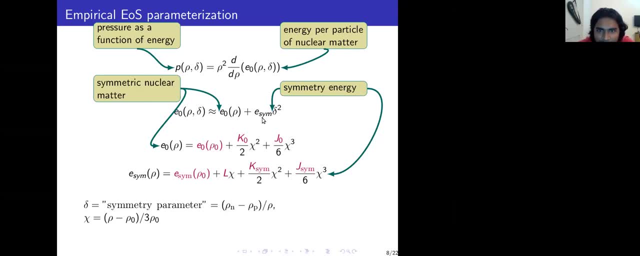 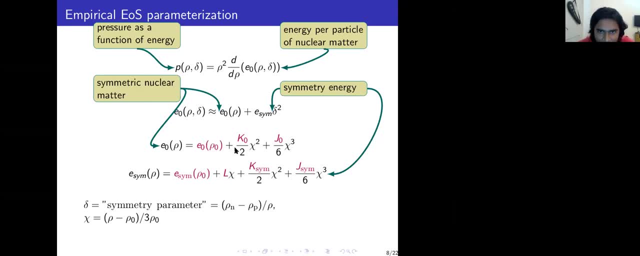 these parameters based on some nuclear physics experiments here? Yes, my question is that. Yeah, I'm coming to that point. So now there are other type of nuclear physics parametrization. So, for example, they are based on chiral effective field theory or relativistic mean field theory. 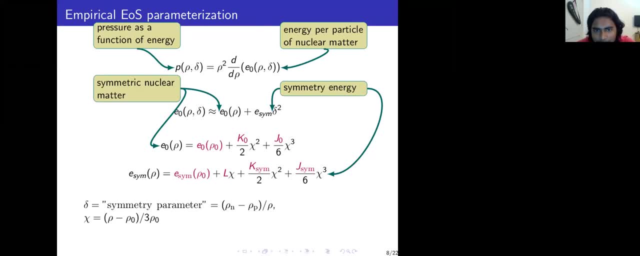 So what they do here? so they treat each neutrons and protons as a relativistic particle, And so now you can imagine them as direct nuclear right, And for that system you can write the Lagrangian of that Lagrangian will be direct Lagrangian. Yes, You can solve the equation of. 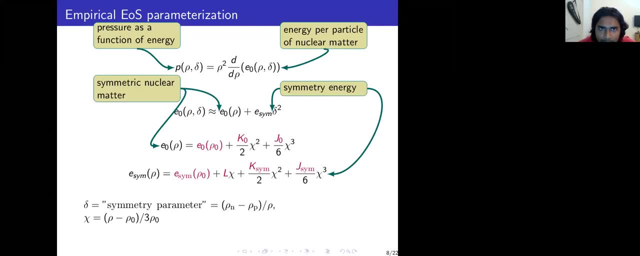 motion and calculate the equation of state. Now, those equations of state can be produced by, by these parameters here. So we can tune our parameters in such a way: you can now produce those parameters. So that's how. so that's the. that is the reason that we are doing it in a 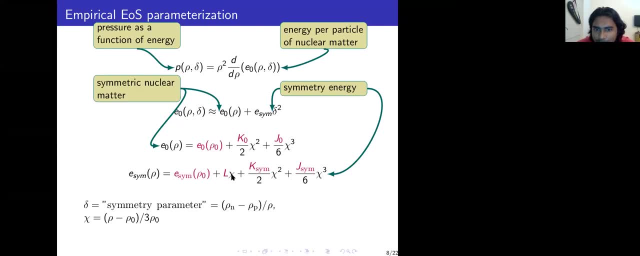 sort of model-independent way. So we do not want to consider any model, but we can actually explain any model by this parametrization. Sorry, just one quick confusion. So from the Lagrangian you get the equation of state or the equation of. So by solving the Lagrangian equation of motion, 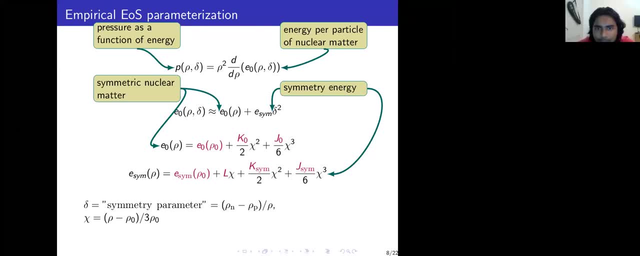 Yes, you get the equation of motion right. Yeah, So from the equation of motion you can calculate the energy pressure also. So that is, that will be the equation of state. Okay, Thank you. Yeah, you're welcome. 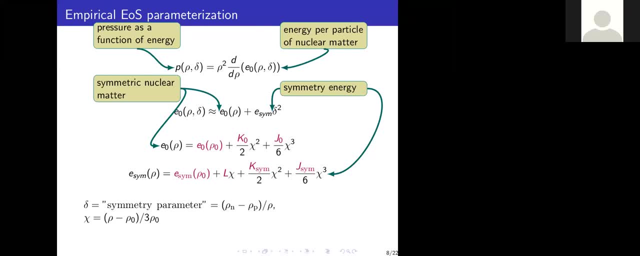 Sir, please go ahead. Okay, So, is this also safe? Yes, sir, But okay, So I I just I'm just my question is: can you? Yes, sir, I thanks you. I think he isband. 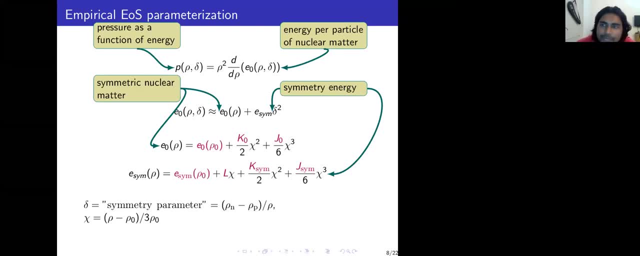 Can you? can you hear me? Yeah, I can hear you. Yes, sir, Okay, So can you just very briefly say that when they're looking at the equation of motion x-ray observation, what are they actually seeing? I mean, what are the observations that are causing? 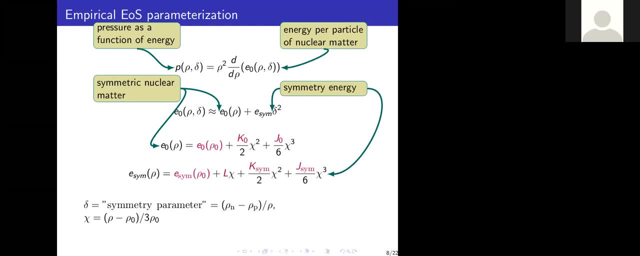 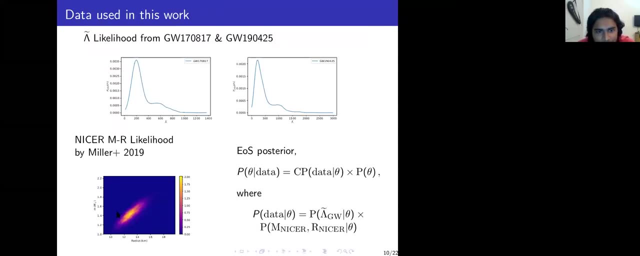 you know, giving these constraints or giving these parameters. So from the x-ray observation actually we get the mass-radius distribution, And this mass-radius distribution depends on the equation of set parameters actually, And so we need any kind of macroscopic properties from the observation. So GW grouping as this: 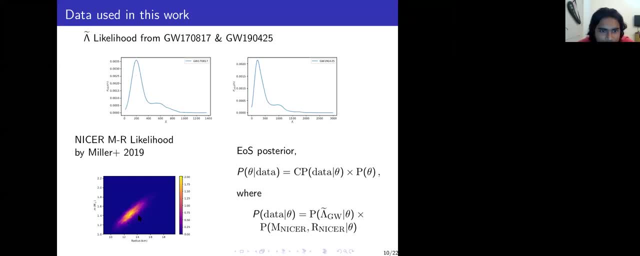 lambda x-ray gives us a mass-radius. So they are looking at the x-ray spectrum or they are looking. So that question. So from the x-ray observation we get the x-ray photons here, And from the luminosity actually we are calculating the mass of the neutron star. 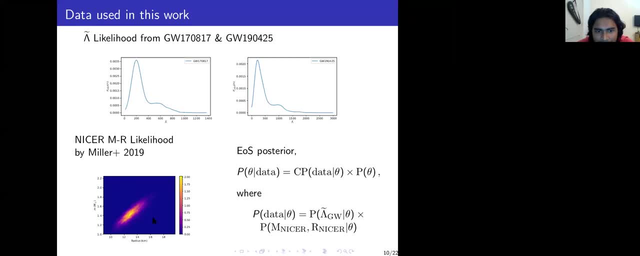 And from the x-ray spectrum. we can calculate the radius of the neutron star from the spectroscopy But the radius measurement is not very reliable from the x-ray because it also involves some modeling about the neutron star atmosphere And that atmosphere modeling is a bit tricky. 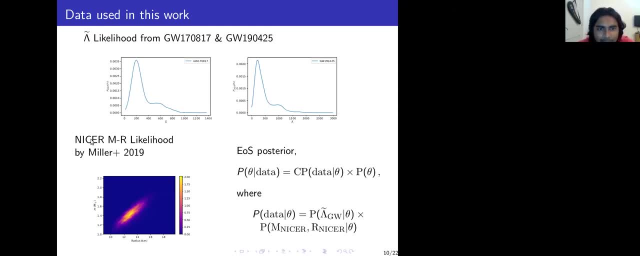 But NYSAR claims that their data is right now strong enough to actually overcome that model dependency. So this is a very accurate measurement they are claiming right now. Thank you, Okay, So there is no more questions. I will ask Essie to go ahead with her question.